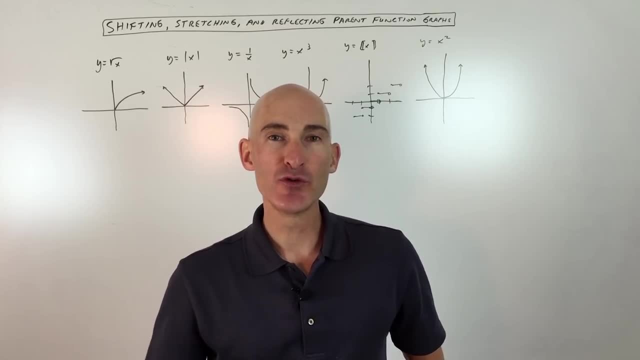 Hi, this is Mario, with Mario's Math Tutoring, coming to you with another math video to help you boost your score in your math class, improve your understanding and, hopefully, make learning math a lot less stressful. So what we're going to talk about in this video is how to stretch, shift, translate, reflect all the different types of transformations that you can do with parent functions. 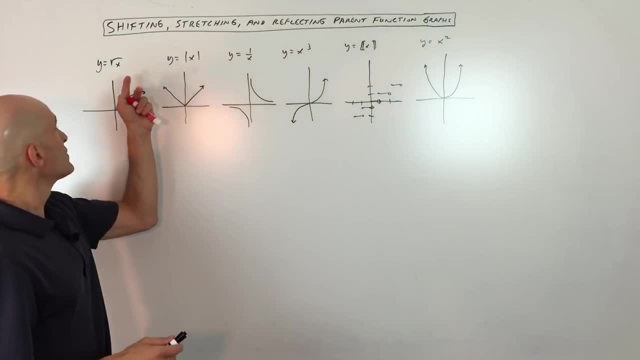 So let's get right into this video and look at some examples. So first of all, you want to familiarize yourself with a lot of these basic graphs If you recognize the basic shape of the graph and the basic equation. that's the starting point. 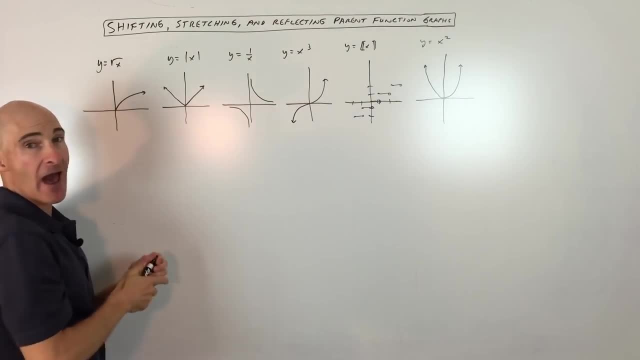 So let's just go through them real quick. This is the square root function and it looks like half a parabola on its side. This is the absolute value function and it looks like a real sharp V with the vertex at the origin. 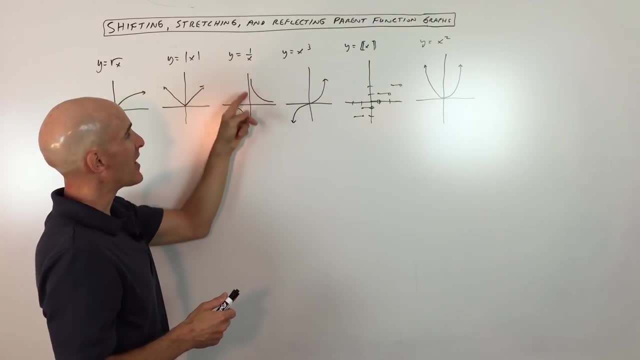 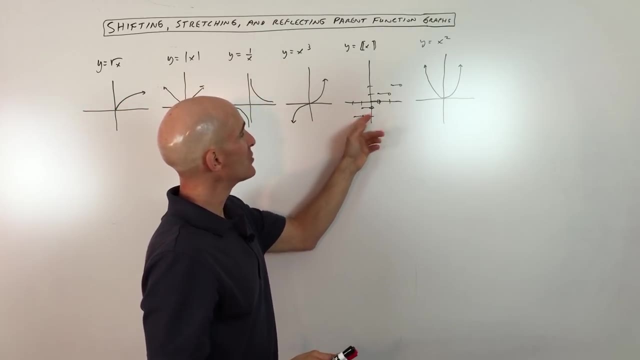 This is called the reciprocal function because it's not x but 1 over x, and you can see it's actually a hyperbola. It approaches the x and y axes. y equals x cubed. This is the greatest integer function. It looks like steps. 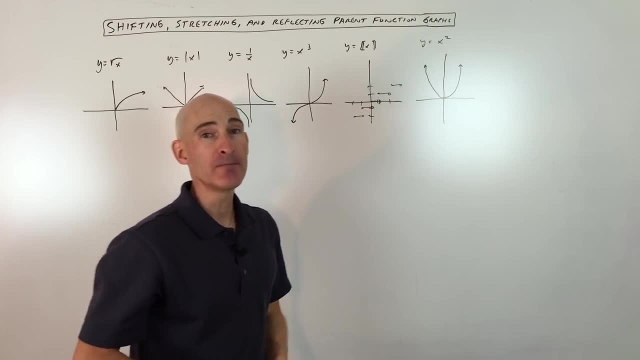 And then, of course, y equals x squared. That's our u-shaped u-shaped graph, our parabola. But now let's talk about transforming these graphs. So let's just start with this one over here: y equals square root of x. 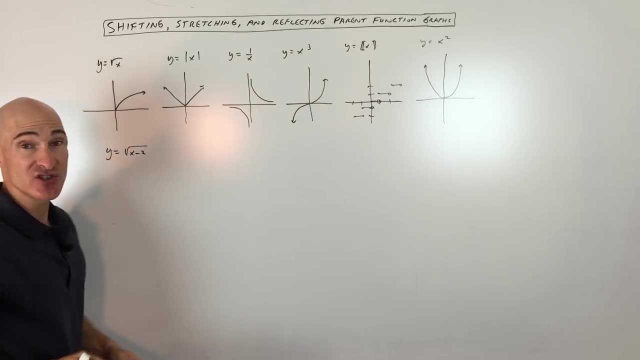 Say, for example, we wanted to graph: y equals square root of x minus 2.. What do you think that 2 does to the graph? Well, if you said shift's right, you're right. Basically, the way you want to think about it is: whatever number is grouped with, the x is going to shift the graph okay, in the x direction. 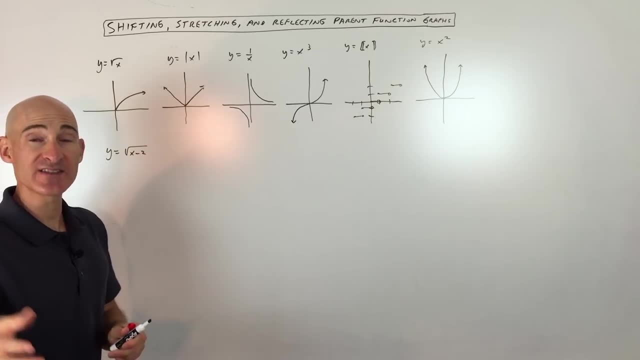 It's going to affect the x or the horizontal direction, But it's the opposite from. you know what it initially looks like. So if it's minus 2, it actually shifts it right, positive 2.. If this was plus 2, it actually would shift left 2.. 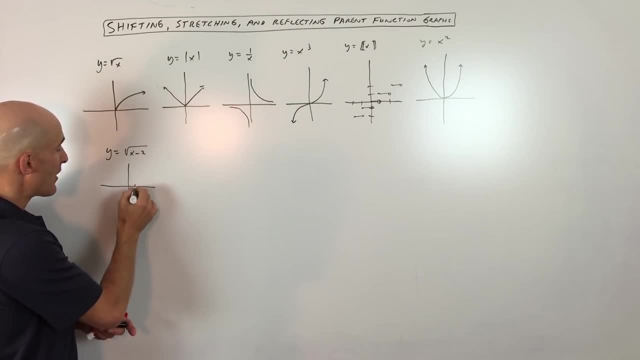 So, just to show you on this graph here, this is actually going to be shifting our graph right. 1,, 2, and there's our graph. Okay, so are you with me so far? Let's look at another example. Let's say we have y equals absolute value of x. okay, 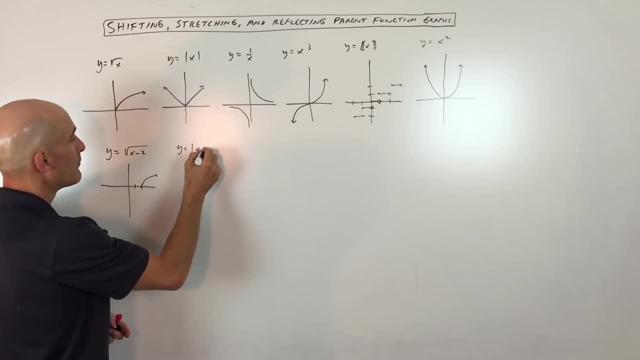 Say we wanted to graph, y equals x plus 3.. So what do you think the plus 3 does to the, to the graph, the parent function? Okay, if you said shift's left 3, you're right. Okay, and again, notice how see it's grouped with the x, right. 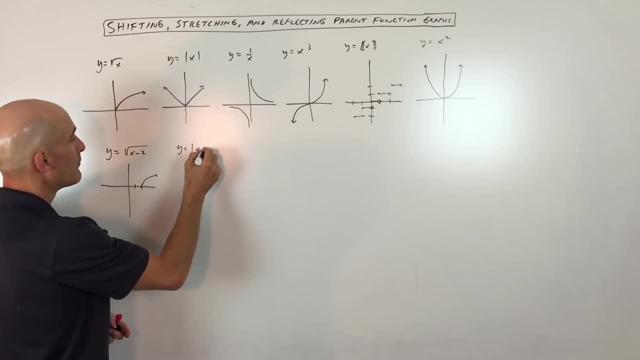 Say we wanted to graph, y equals x plus 3.. So what do you think the plus 3 does to the, to the graph, the parent function? Okay, if you said shift's left 3, you're right. Okay, and again, notice how see it's grouped with the x, right. 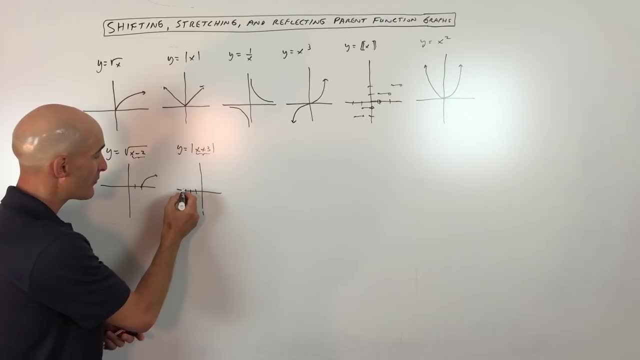 It's grouped with the x, but it's having the opposite effect. It's actually shifting the graph left- 3.. So now the vertex is over here at negative 3.. Everything shifted left 3.. Okay, let's go to the next graph. y equals 1 over x. 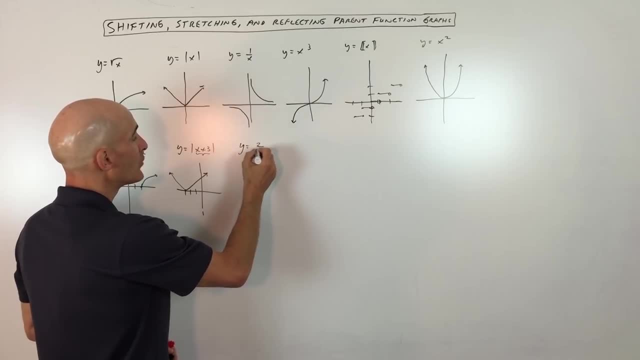 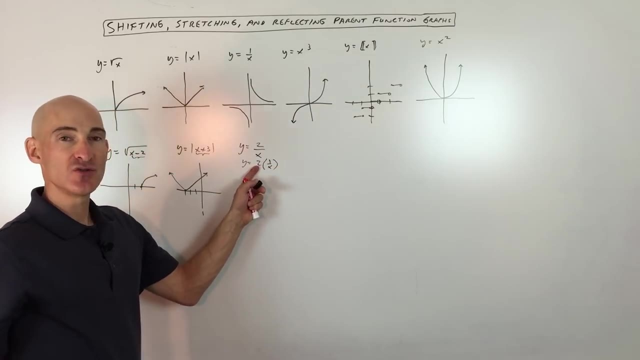 What we're going to do now is we're going to multiply okay by 2.. So basically, what I did is I said this is 2 times 1 over x. What do you think the 2 does to this graph? If you said vertical shift, not vertical shift, I'm sorry, vertical stretch. 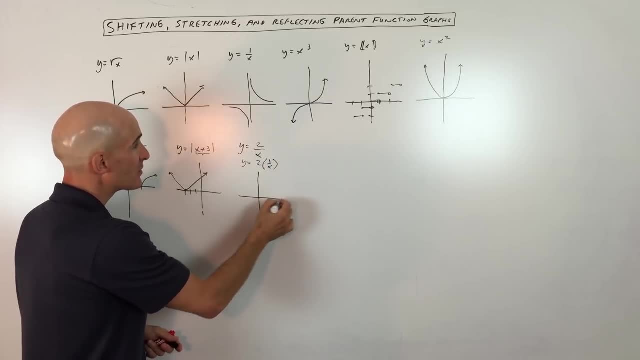 meaning you're multiplying all the y values by 2,. you're exactly right, And so what would happen is: normally this graphic goes through the point 1, 1.. Okay, you can see, if you put 1 in here, that's 1.. 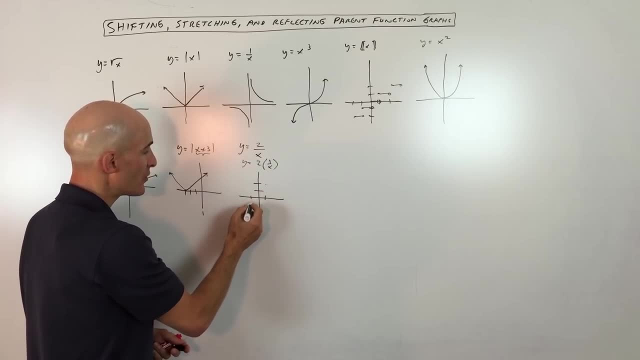 But now it's going to be stretching. It's going to be up here at 2.. Same thing over here at negative 1.. It's going to be at negative 2.. So what's happening is: okay, it's a vertical stretch. 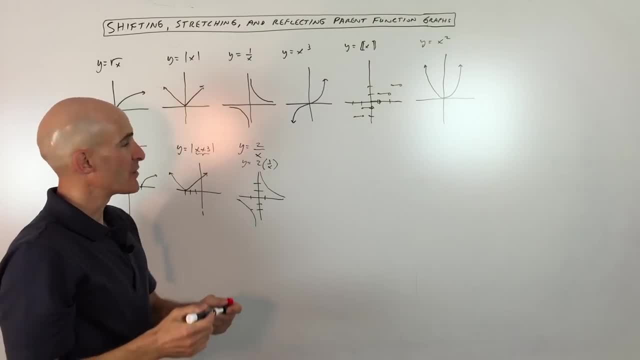 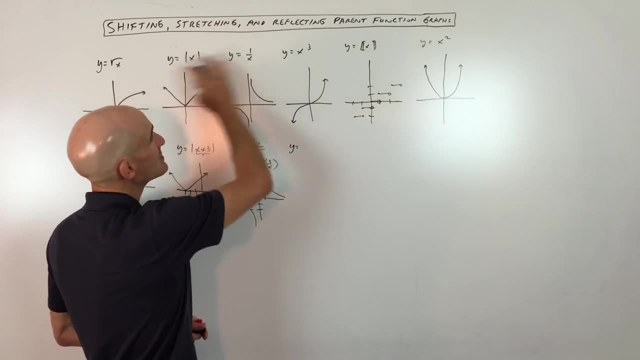 Like you pulled on it, It's going to be up in this direction. Okay, now hang in there with me. I'm going to show you some general concepts. Let's go to the next one. here, y equals x cubed. Now what you can do is you can write any of these parent functions in a more general way. 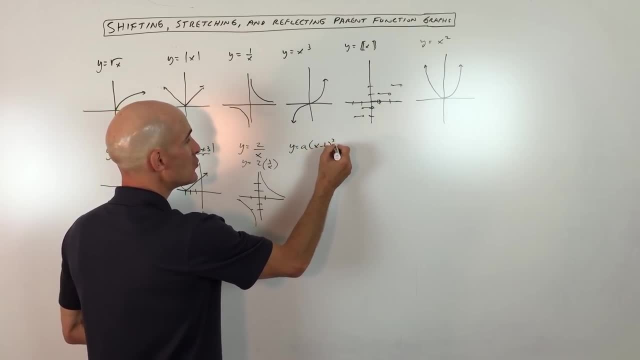 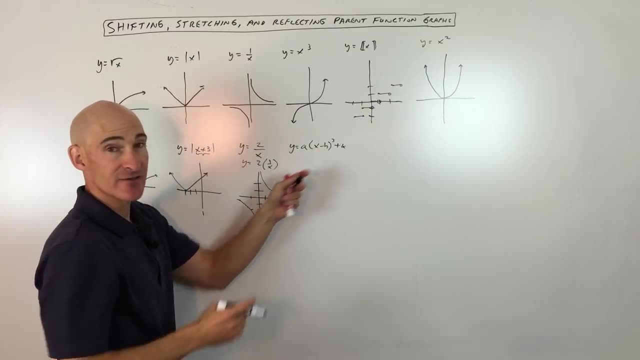 like this: y equals a x minus h, cubed plus k. So what we've already kind of, you know, gotten familiar with here is that the number that's grouped with the x is affecting the x direction right. If it's minus 2, it's shifting right 2.. 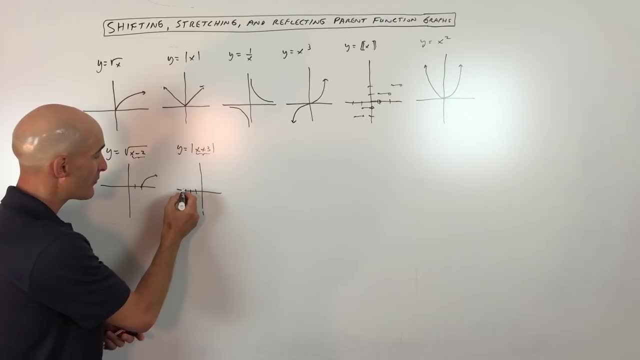 It's grouped with the x, but it's having the opposite effect. It's actually shifting the graph left- 3.. So now the vertex is over here at negative 3.. Everything shifted left 3.. Okay, let's go to the next graph. y equals 1 over x. 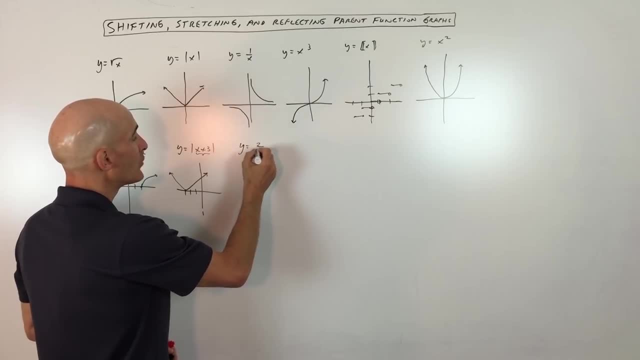 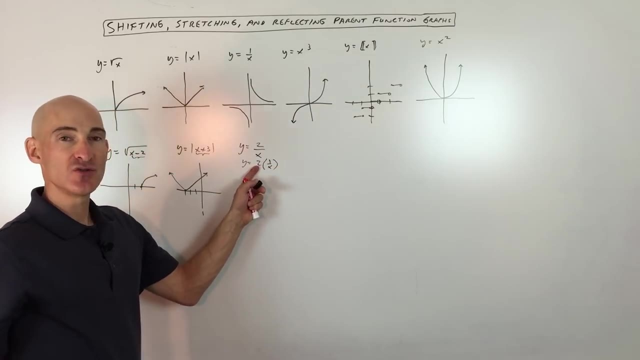 What we're going to do now is we're going to multiply okay by 2.. So basically, what I did is I said this is 2 times 1 over x. What do you think the 2 does to this graph? If you said vertical shift, not vertical shift, I'm sorry, vertical stretch. 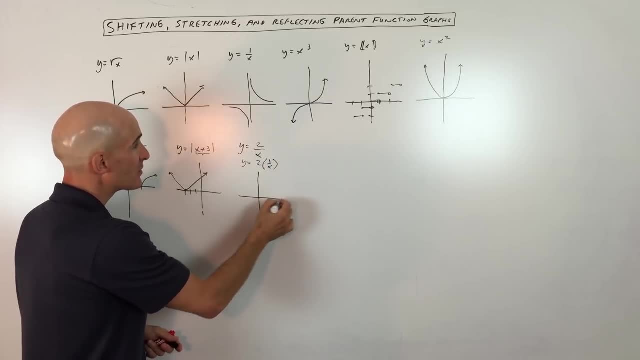 meaning you're multiplying all the y values by 2,. you're exactly right, And so what would happen is: normally this graphic goes through the point 1, 1.. Okay, you can see, if you put 1 in here, that's 1.. 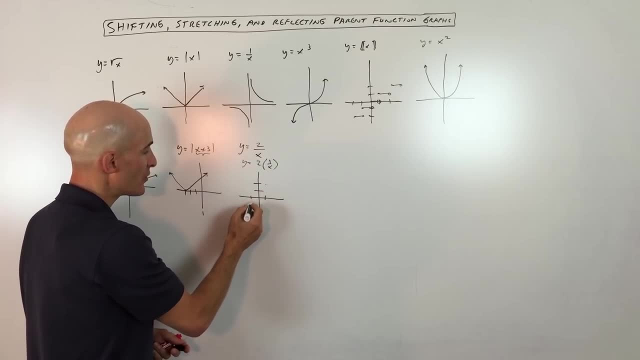 But now it's going to be stretching. It's going to be up here at 2.. Same thing over here at negative 1.. It's going to be at negative 2.. So what's happening is: okay, it's a vertical stretch. 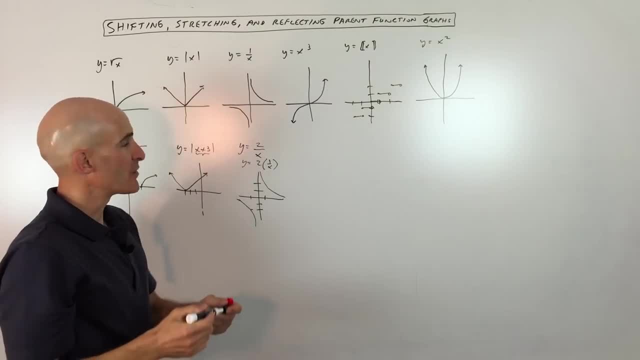 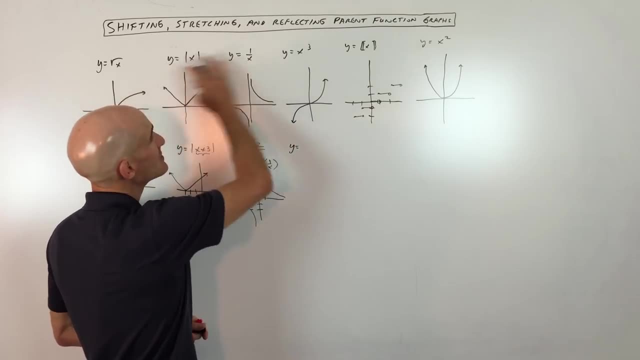 Like you pulled on it. It's in this direction. Okay, now hang in there with me. I'm going to show you some general concepts. Let's go to the next one. here, y equals x- cubed. Now what you can do is you can write any of these parent functions in a more general way, like this: 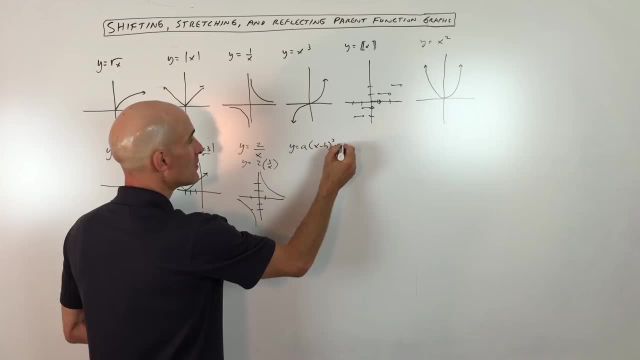 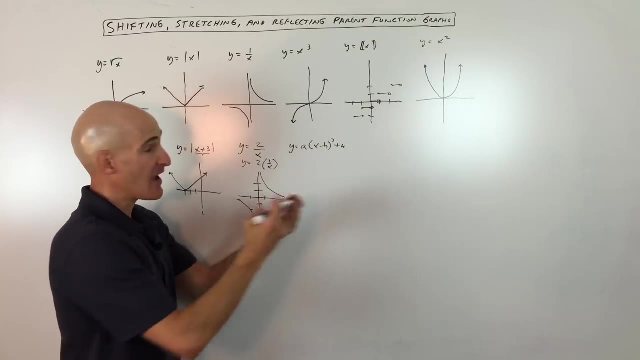 y equals a x minus h cubed plus k. So what we've already kind of, you know, gotten familiar with here is that the number that's grouped with the x is affecting the x direction right. If it's minus 2, it's shifting right 2.. 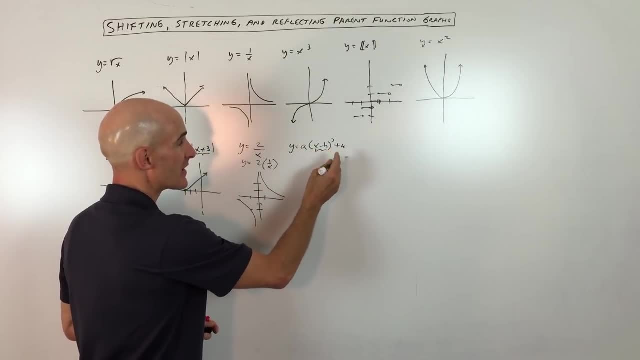 If it's plus 2, it's left 2.. The one that's grouped with the x has the opposite. This k value here has the same effect. If you add 2 to the graph, it's going to shift it up 2.. 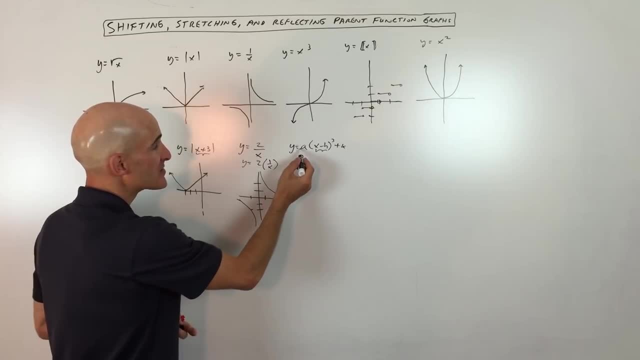 If you subtract 2, it's going to shift it down 2.. And then this number here in front, the a, is going to stretch it vertically. Or if it's less than 1,, like a half or a third, it's going to compress it. 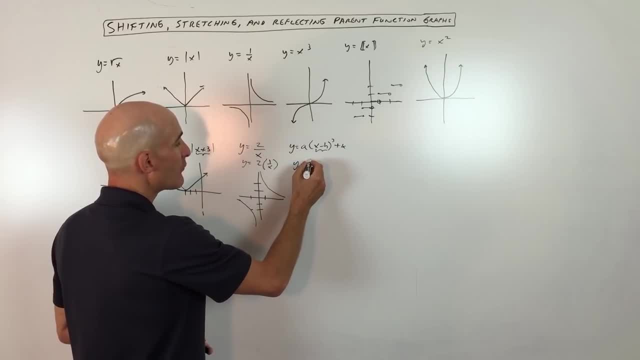 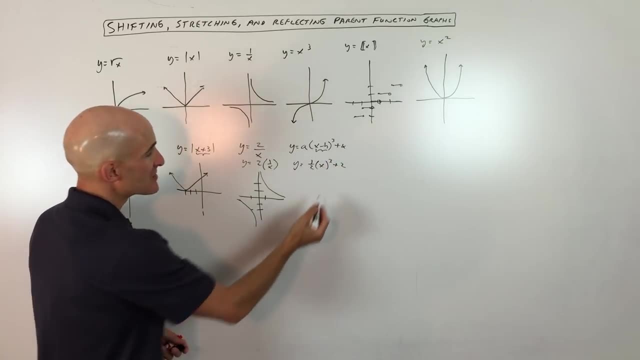 Okay, so you're with me so far. So let's look at an example. Let's say we wanted to graph. y equals 1 half x cubed plus 2.. All right, so what we can see here is that we're going to be multiplying. 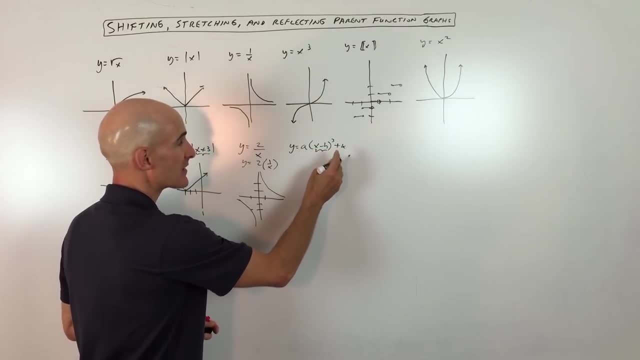 If it's plus 2, it's left 2.. The one that's grouped with the x has the opposite. Okay, It has the opposite effect. This k value here has the same effect. If you add 2 to the graph, it's going to shift it up 2.. 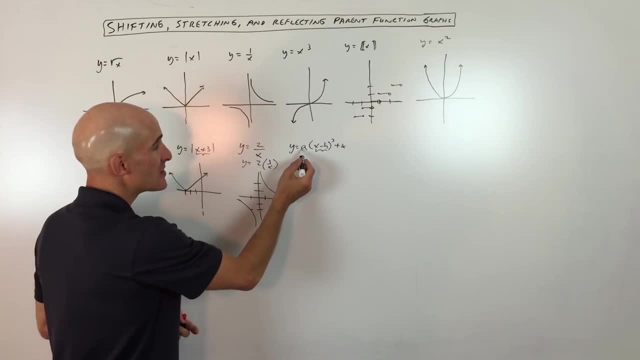 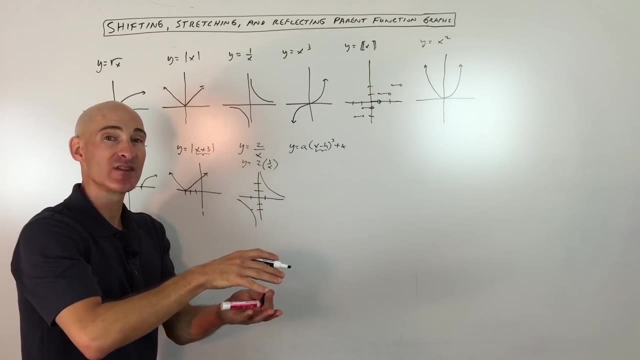 If you subtract 2, it's going to shift it down 2.. And then this number here in front, the a, is going to stretch it vertically. Or if it's less than 1,, like a half or a third, it's going to compress it. 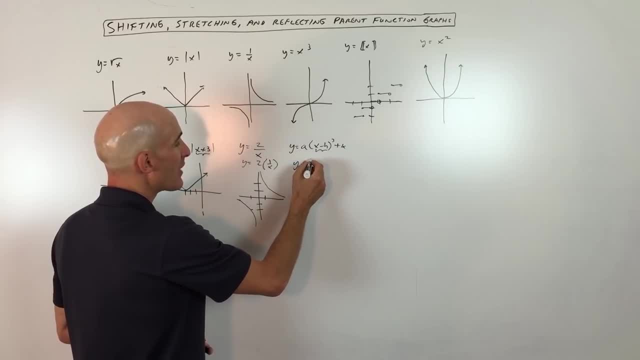 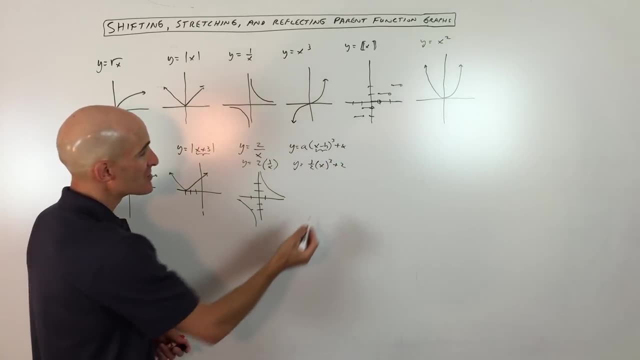 Okay, So you're with me so far. So let's look at an example. Let's say we wanted to graph: y equals 1 half x cubed plus 2.. All right, So what we can see here is that we're going to be multiplying. 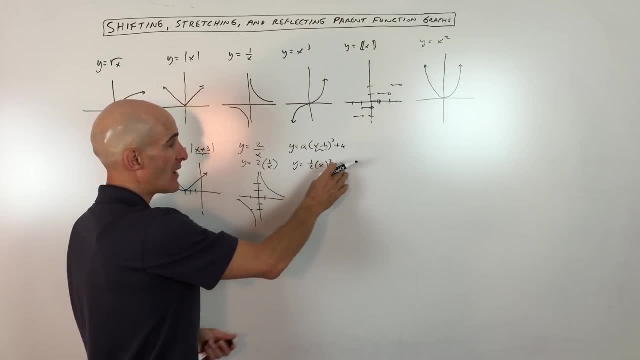 Multiplying the y values by 1 half. so that's a vertical compression and we're going to be picking up the graph and shifting it up 2.. Now, what a lot of students will do okay and a lot of teachers will recommend, is they'll. 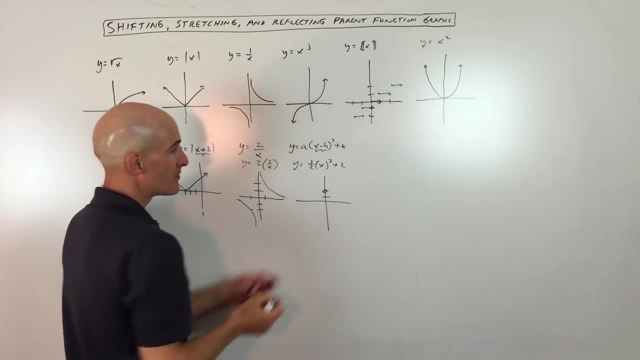 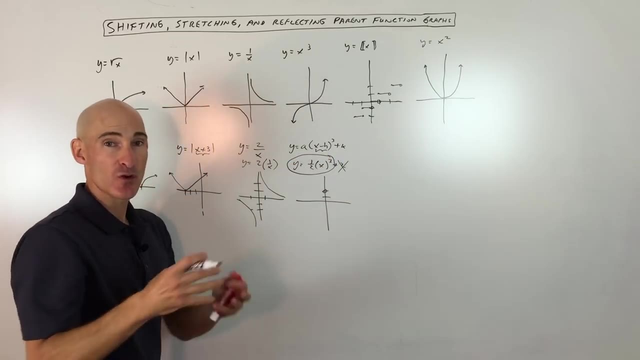 say: okay, we know this is shifting up 2, so let's think of this point here as our starting point. So we've taken the 2 into account. What we'll do now is we'll focus in on this core function here and we're going to make 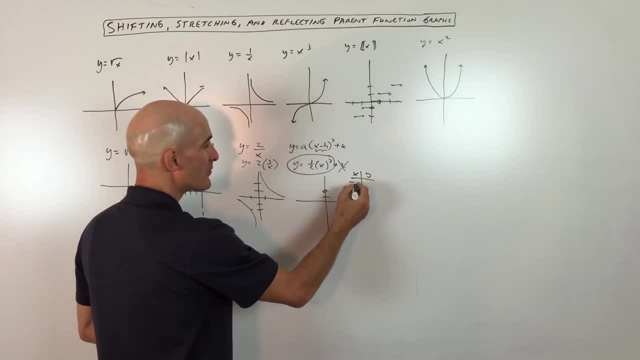 a table of values. So we're just going to say, like x and y, we're going to pick some easy values, right? So if I put negative 1, that's negative 1. cubed Y equals 1 half is negative 1 half. 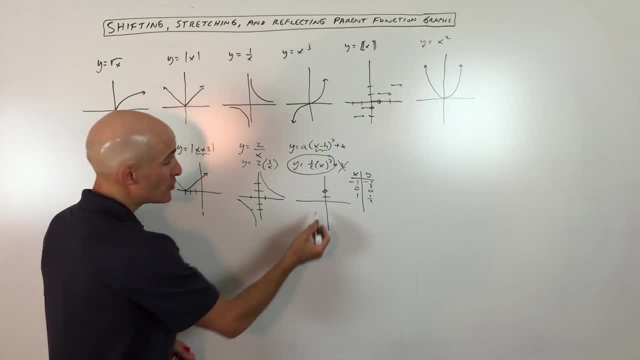 1 would be a positive 1 half and 0 would be 0.. But what you're going to do? instead of graphing from the origin, you're going to treat this point like the origin. So here's: 0, 0.. 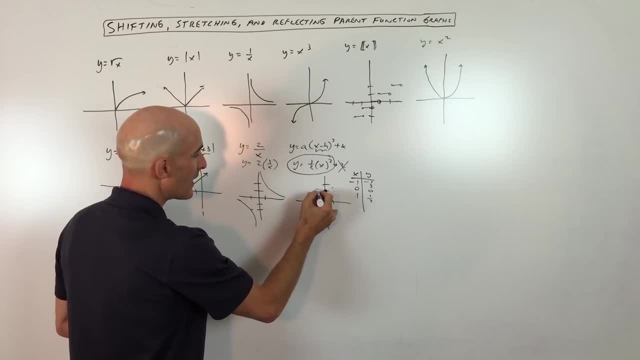 Here's 1, 1 half and here's negative 1, negative 1 half. So now the graph looks like this and what you can see is it's been compressed and it's been shifted up. 2, okay. 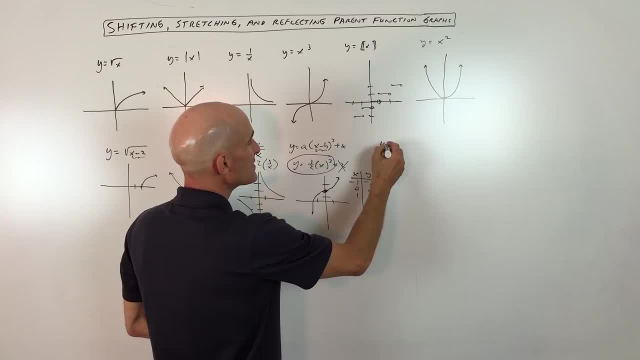 Let's look at another example. Let's take a look at this step function here. Say we wanted to graph: y equals 1.. Y equals negative. okay, Now again, you're probably seeing the pattern. okay, Here we're multiplying everything by negative 1, so what does that do to the y values? 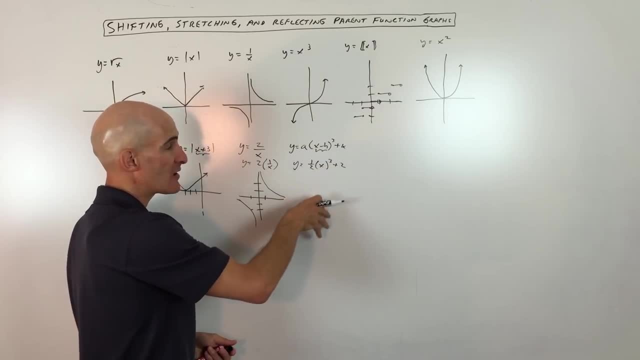 We're multiplying the y values by 1 half, so that's a vertical compression, And we're going to be picking up the graph and shifting it up 2.. Now what a lot of students will do okay and a lot of teachers will recommend. 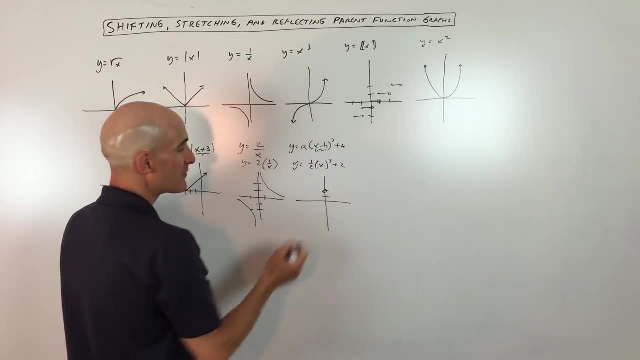 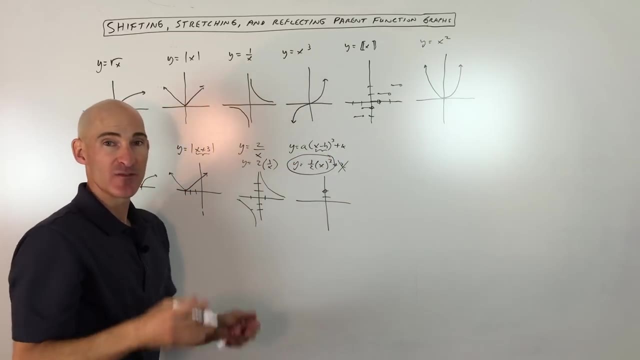 is. they'll say: okay, we know this is shifting up 2.. So let's think of this point here as our starting point. So we've taken the 2 into account. What we'll do now is we'll focus in on this core function here. 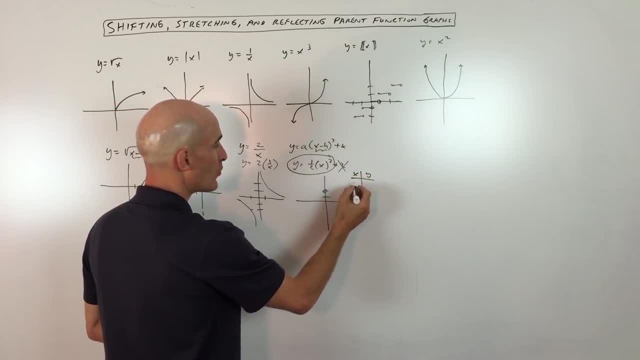 And we're going to make a table of values. So we're just going to say, like x and y, We're going to pick some easy values, right? So if I put negative 1, that's negative 1 cubed times 1 half. 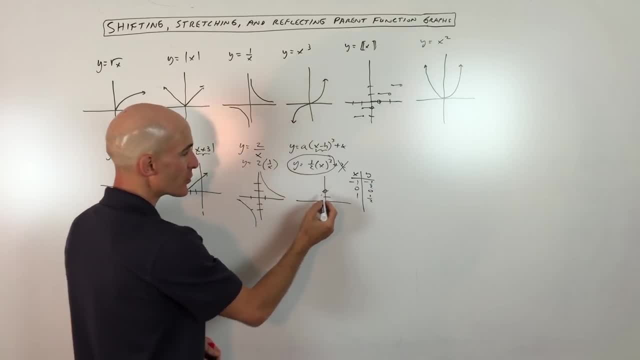 If it's negative, 1 half, 1 would be a positive 1 half and 0 would be 0. But what you're going to do, instead of graphing from the origin, you're going to treat this point like the origin. 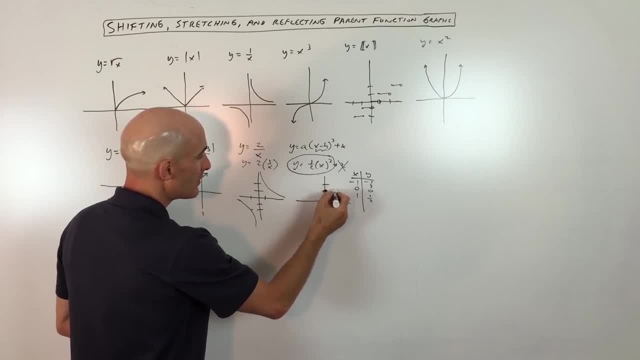 So here's 0, 0.. Here's 1, 1 half And here's negative 1, negative 1 half. So now the graph looks like this And what you can see is it's been compressed and it's been shifted up 2.. 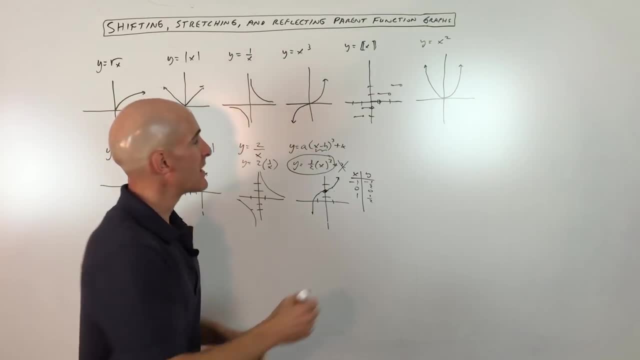 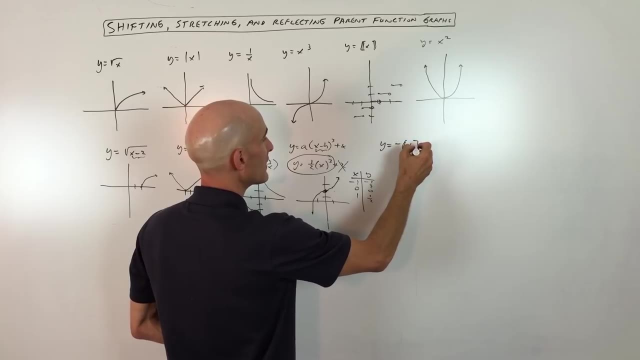 Okay, Let's look at another example. Let's take a look at this step function here. Say we wanted to graph: y equals Negative. Okay, Now again you're probably seeing the pattern. Okay, Here we're multiplying everything by negative 1.. 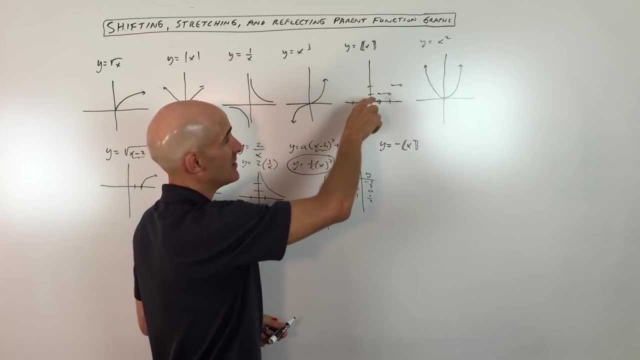 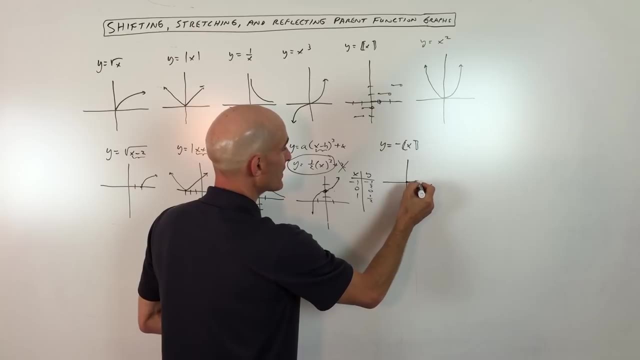 So what does that do to the y values? It makes them the opposite. So it's reflecting over the x-axis. Okay, So now what will happen with this graph is, instead of the stairs going like, so okay, they're going to be reflecting over the x-axis. 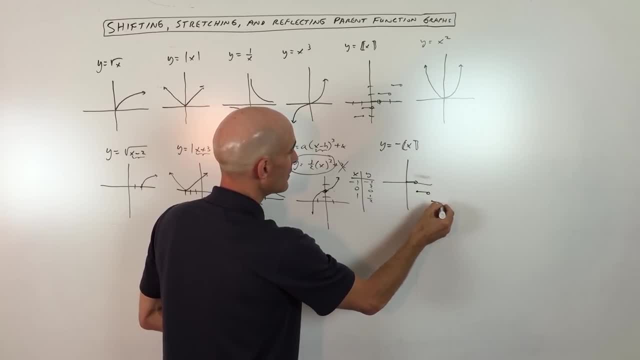 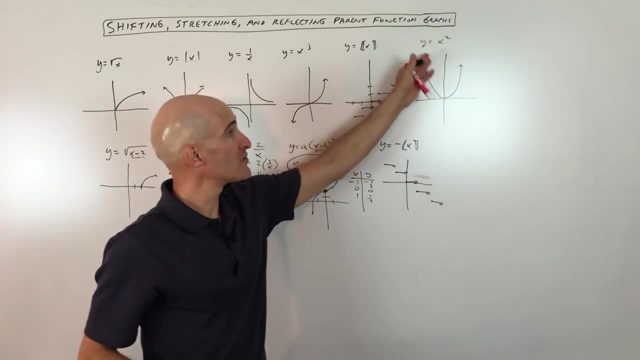 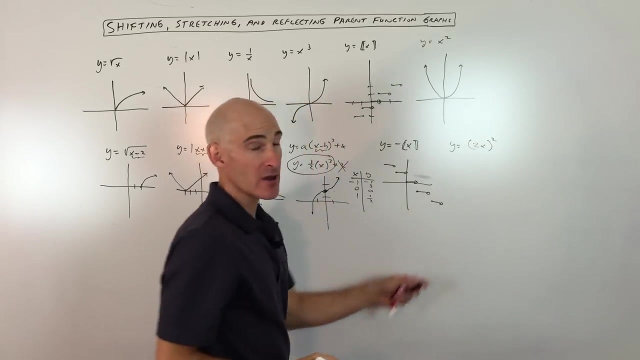 and they're going to be going this direction. Okay, And these ones are going to be up here. Okay, are you with me? so far? Okay, let's look at y equals x squared. Let's say we wanted to graph: y equals 2x squared. 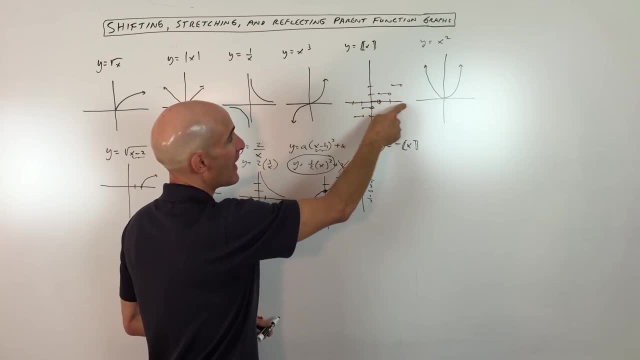 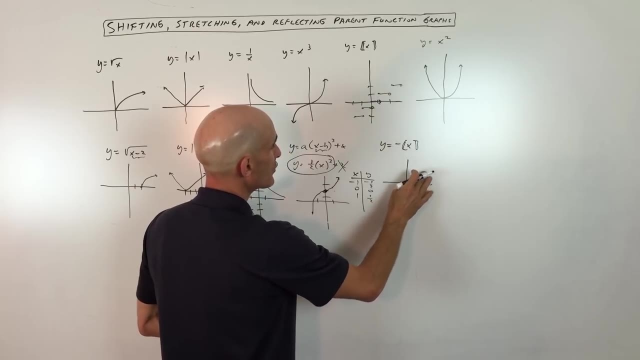 It makes them the opposite. so it's reflecting over the x axis. okay, So now what will happen with this graph is, instead of the stairs going like, so okay, they're going to be reflecting over the x axis and they're going to be going this direction. 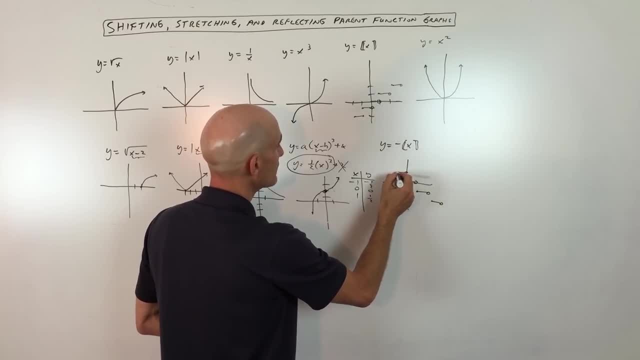 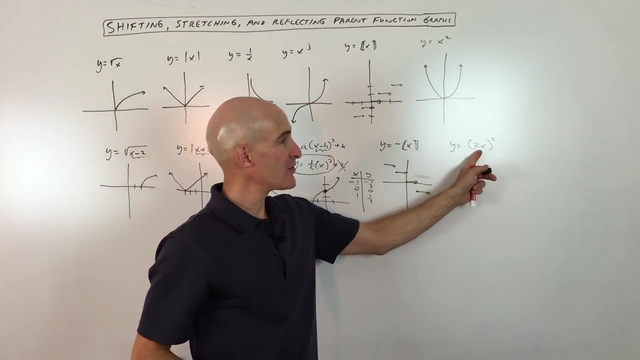 okay, And these ones are going to be up here. Okay, are you with me so far? Let's look at y equals x squared. Let's say we wanted to graph y equals 2x squared. Now the thing to pay attention to is, you see, how the 2 is grouped with the x. 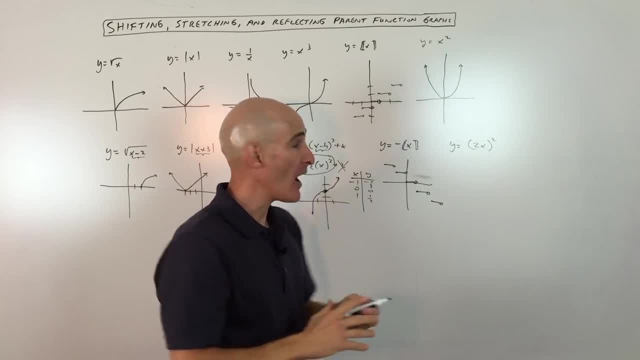 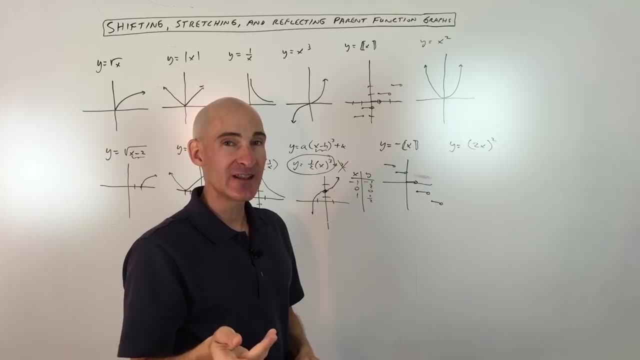 When it's grouped with the x, it affects the x direction, but in the opposite fashion. okay, However, you want to say that. So basically, instead of multiplying the x's by 2, you're actually going to be dividing them by 2.. 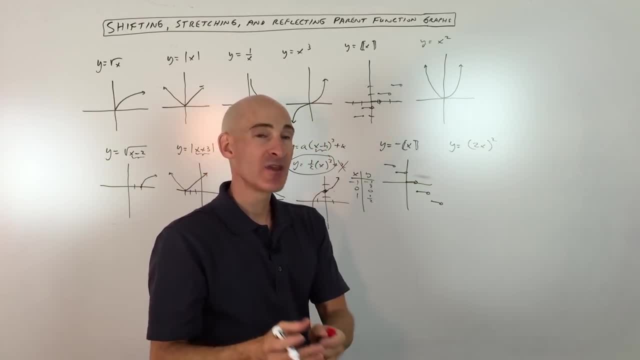 Now the thing to pay attention to is: you see how the 2 is grouped with the x. When it's grouped with the x, it affects the x direction, but in the opposite fashion. Okay, However, you want to say that. So basically, instead of multiplying the x's by 2, you're actually going to be dividing them by 2.. 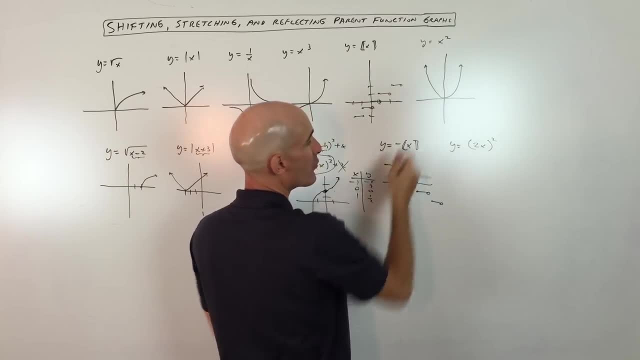 So what happens is this is actually f going to be a horizontal compression. okay, so basically what's going to happen here is: normally the graph goes through 0, 0, 1, 1, but now it's going to be 1 half 1 and negative 1 half 1. so basically what we did is we compressed it that way. 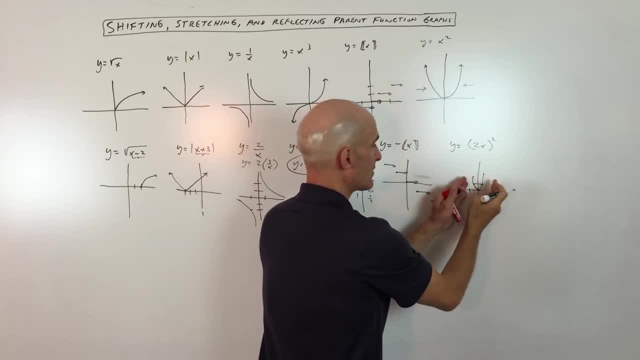 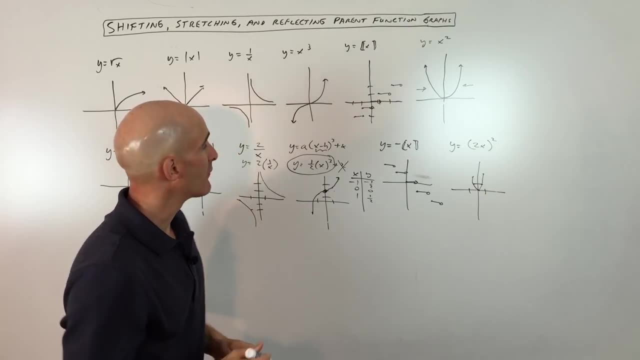 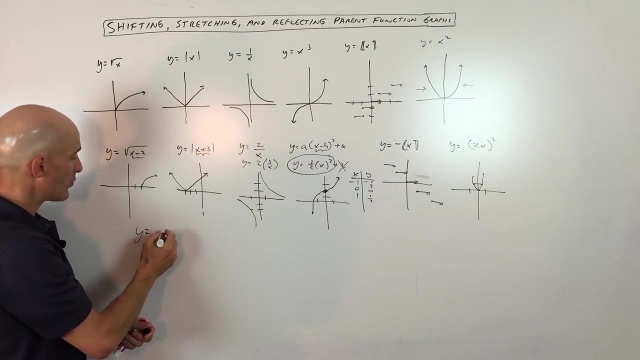 and you can see it's like being squished right, okay, horizontally. so let's look at some other examples now I want to make a little bit more challenging for you. so let's say, for example, like: say: for example, you took back to the square root of X function. say we wanted a graph: y equals 3 square root of x plus 2 minus 1. 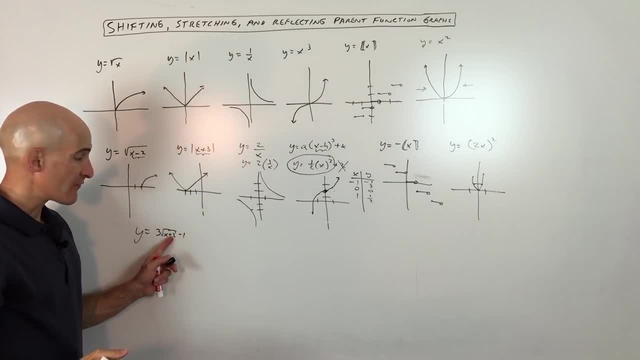 okay, so you can see that this is actually going to shift the graph left to. it's going to be a vertical stretch by 3 and then it's going to be shifted down one. now, the reason I did it that way is because I'm following the order. 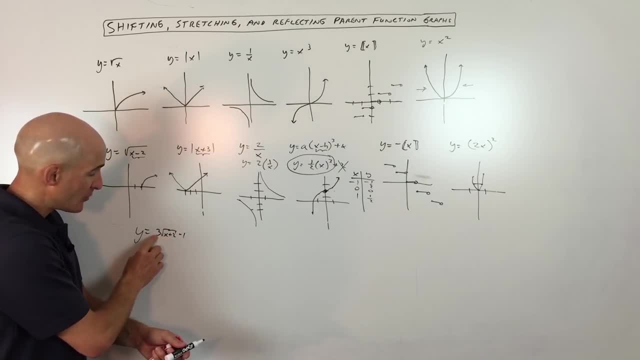 of operations. parentheses, exponents, multiplication, division, addition, subtraction, or you can use multiplication, division, addition subtraction, or you can can think about working from the inside out, okay, but I think about the order of operations. so if you wanted to do this kind of like in slow mo, okay, right, slow. 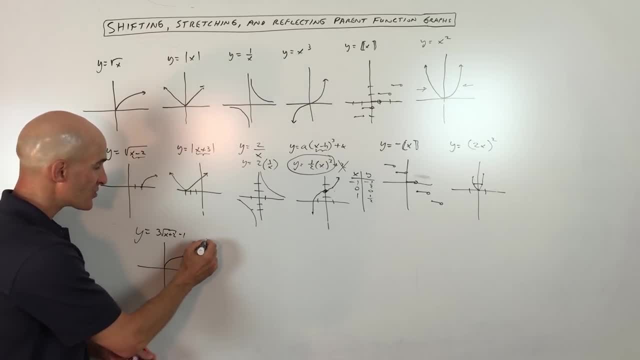 motion. you start with the basic graph here. okay, now you might say to yourself, Mario, I don't know the basic graph, well, just go ahead and make a table, okay, just using that core graph, and pick some values. 0, the square root of 0 is 0, 1 is 1, 4 is 2. 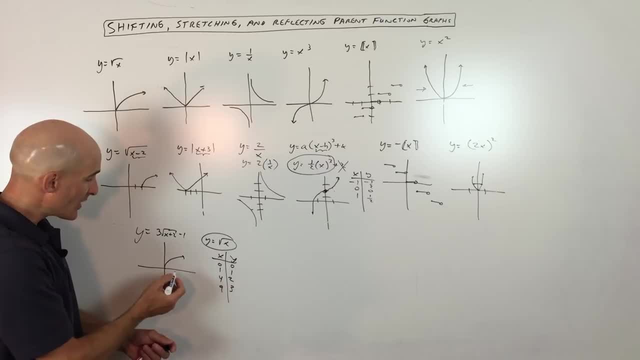 9 is 3. these are your basic points, okay, so then you can plot those. and then you say, hmm, I'm going to subtract 2 from all the X coordinates. so if I subtract 2 from these now, I'll be at negative 2: 0. okay, I'm going to be at negative 1: 1, okay. 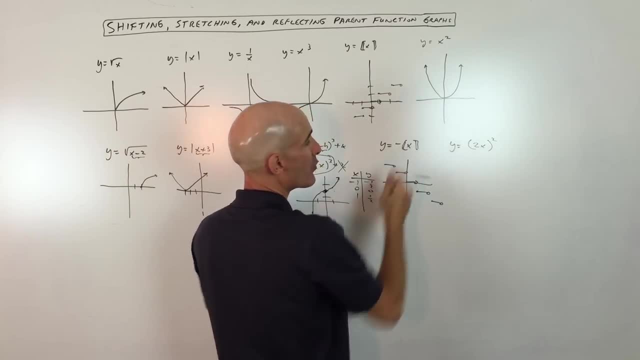 So what happens is this is actually going to be A horizontal compression. Okay, so basically, what's going to happen here is: normally the graph goes through 0, 0, 1, 1.. But now it's going to be 1 half 1 and negative 1 half 1.. 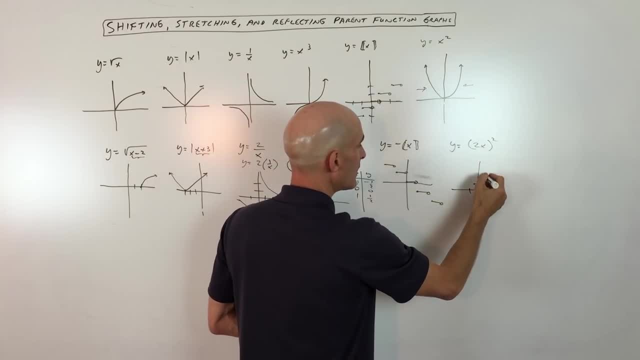 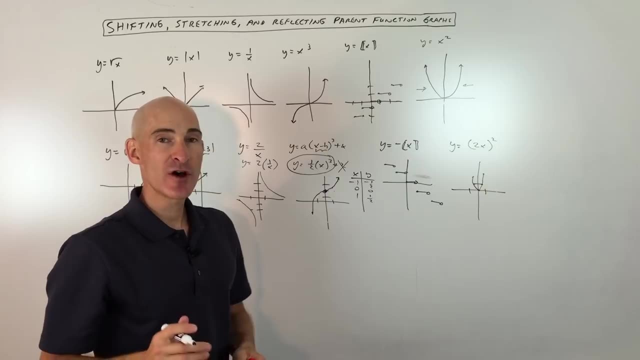 So basically, what we did is we compressed it that way And you can see it's like being squished right- Okay, horizontally. So let's look at some other examples. now I want to make it a little bit more challenging for you. 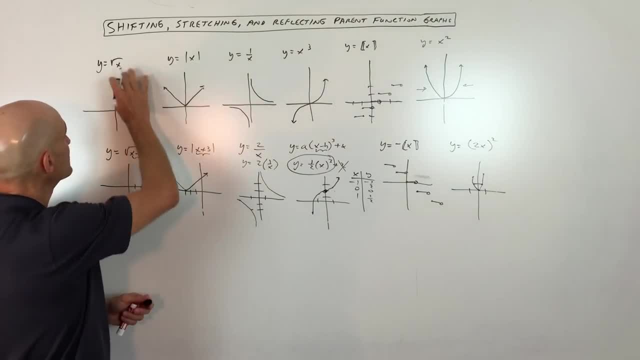 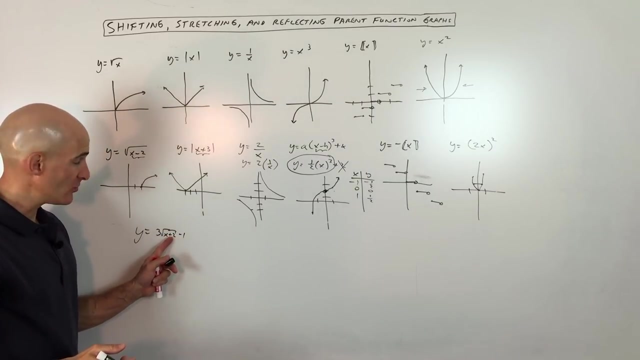 So let's say, for example, like: say: for example, you took back to the square root of x function. Say we wanted to: graph y equals 3 square root of x plus 2 minus 1.. Okay, so you can see that this is actually going to shift the graph left 2.. 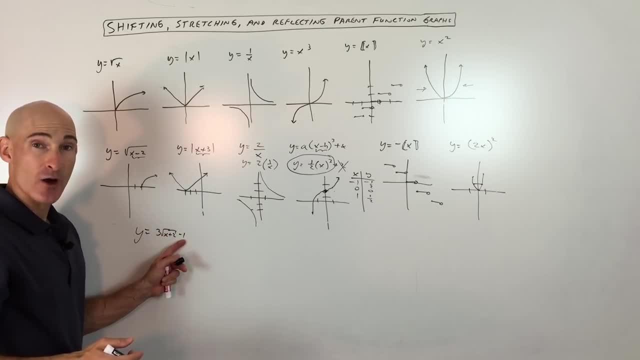 It's going to be a vertical stretch by 3, and then it's going to be shifted down 1.. Now, the reason I did it that way is because I'm following the order of operations- Parentheses. exponents, multiplication, division, addition, subtraction. 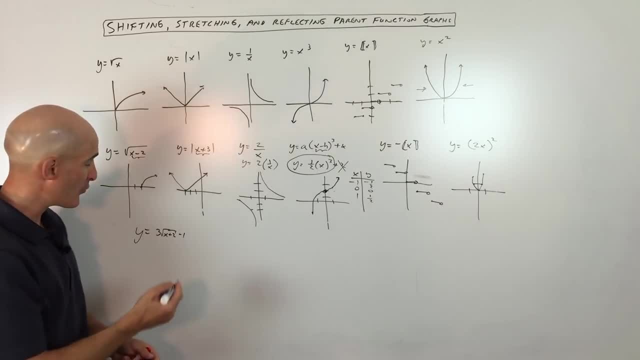 Or you can think about working from the inside out. Okay, But I think about this, I think about the order of operations. So if you wanted to do this kind of like in slow-mo, okay, right, slow motion. you start with the basic graph here. 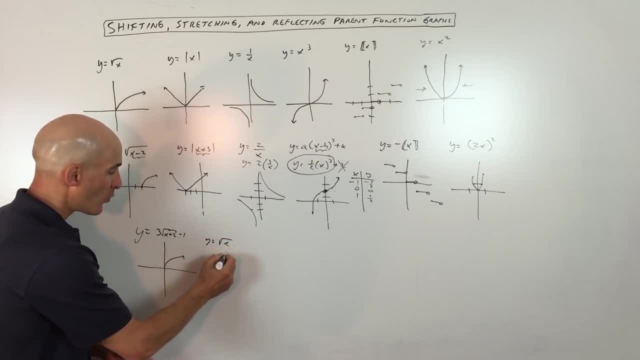 Okay, now you might say to yourself: Mario, I don't know the basic graph, Well, just go ahead and make a table, okay, just using that core graph, and pick some values: 0, the square root of 0 is 0,, 1 is 1,, 4 is 2,, 9 is 3.. 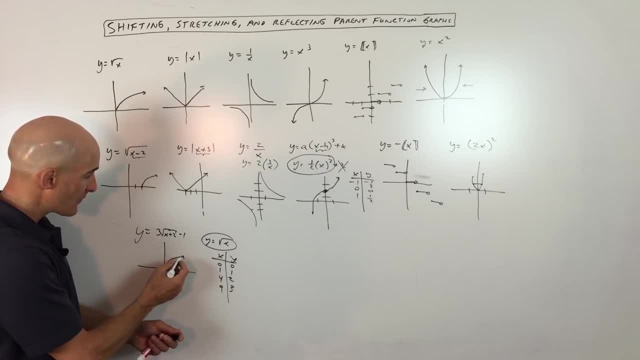 These are your basic points. Okay, so then you can plot those. And then you say: hmm, I'm going to subtract 2 from all the x coordinates. If I subtract 2 from these now, I'll be at negative 2, 0.. Okay, so then you can plot those. And then you say, hmm, I'm going to subtract 2 from all the x coordinates. So if I subtract 2 from these now, I'll be at negative 2, 0.. Okay, so then you can plot those. And then you say, hmm, I'm going to subtract 2 from these now, I'll be at negative 2, 0.. 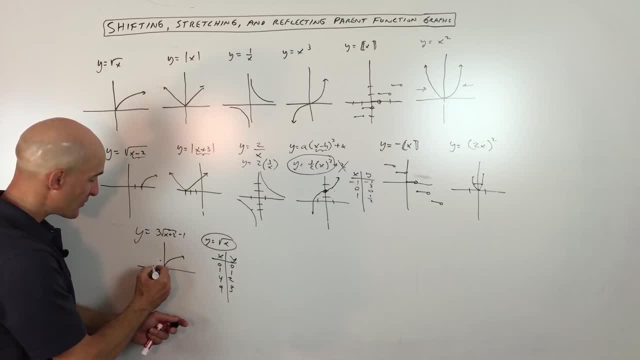 Okay, I'm going to be at negative 1, 1.. Okay, so now I can see my graphs looking something like this: It shifted left: 2.. Now I'm going to be taking all the y values and multiplying by 3.. 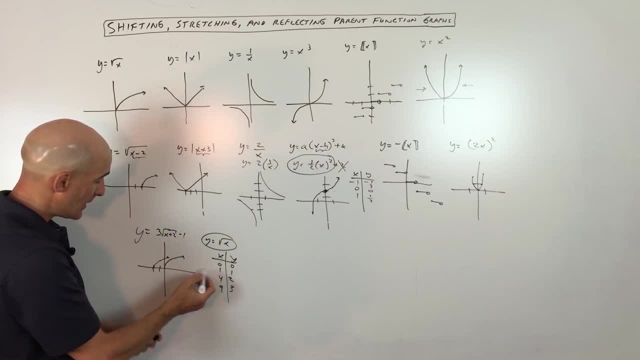 This is a vertical stretch, So instead of being at, you know, negative 1, 1,, I'm going to be at negative 1, 3.. So this point right here is actually going to be moving up 1,, 2, 3.. 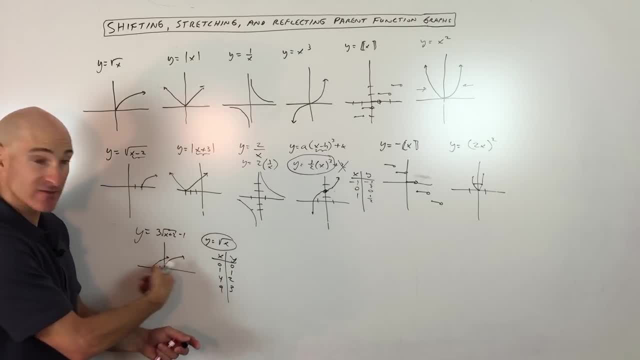 and so now I can see my graphs looking something like like this: shifted left: 2. now I'm going to be taking all the Y values and multiplying by 3. this is a vertical stretch, so instead of being at, you know, negative 1, 1, I'm going to be at. 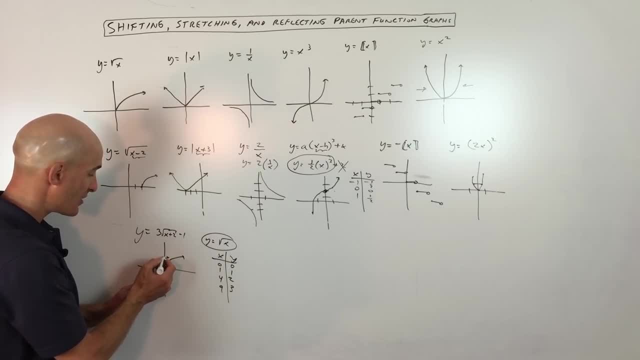 negative: 1, 3. so this point right here is actually going to be a moving up: 1, 2, 3. it's going to be like this: so this is a vertical stretch, okay, and then I'm going to be shifting the whole thing minus 1 down once we'll be. 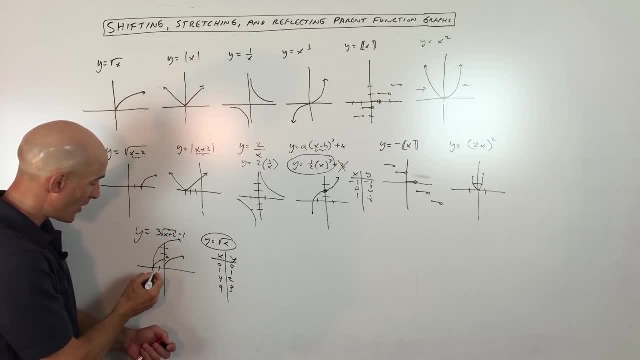 subtracting 1 from all the Y values. so each of these points is going to go down 1, down 1, and so on. so now the graph looks like that. okay, now you might say that sounds like a lot of work, right? so let's do it another way. so this is: 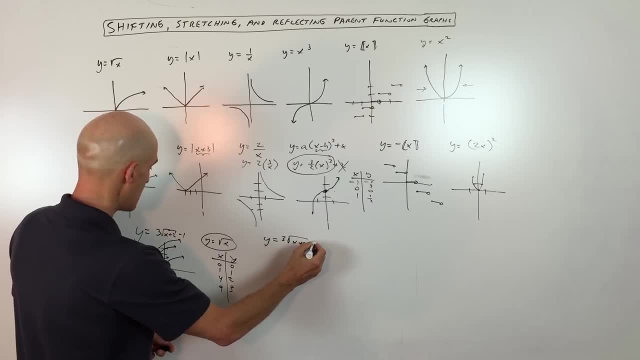 another way that students and teachers will approach it. they'll say: hmm, let's just take the shift into account first. let's just say: okay, we know, this is gonna shift left 2 and down 1 right. so let's just treat that point like our starting point, like our origin. so we've 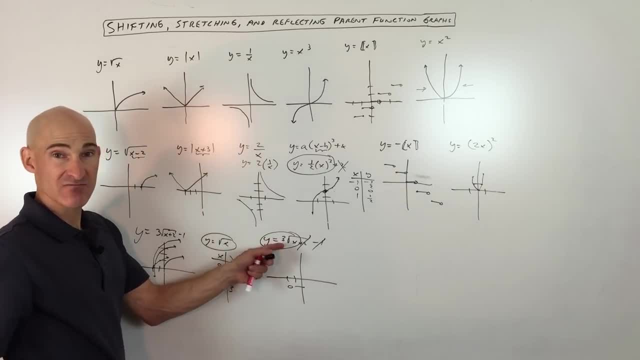 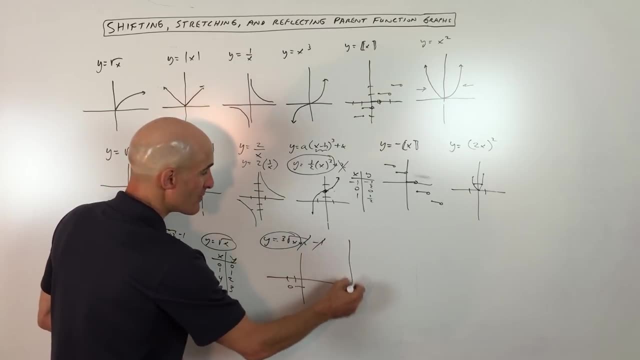 taken those guys into account. now all we have to do is graph this kind of core graph or core equation or core function, but from this point, not the origin. that makes a lot simpler. so you make a table again. pick some easy values that you can take: the square root of 0, 1 & 4. square root 0: 0 times 3 is 0. square root of 1. 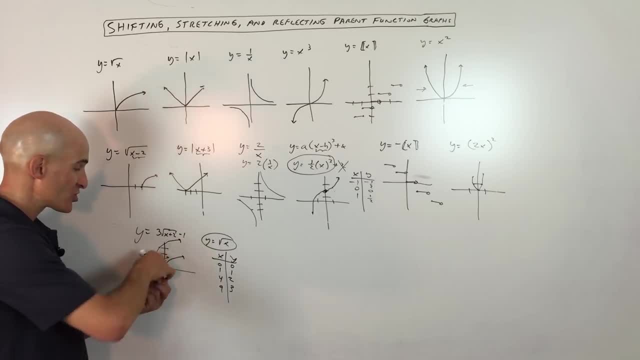 It's going to be like this: So this is a vertical stretch, So this is a vertical stretch, So this is a vertical stretch, okay, and then I'm going to be shifting the whole thing minus one down once, maybe subtracting one from all the Y values. so each of these points is going: 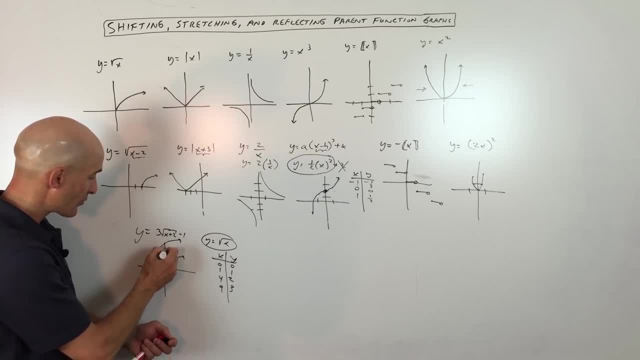 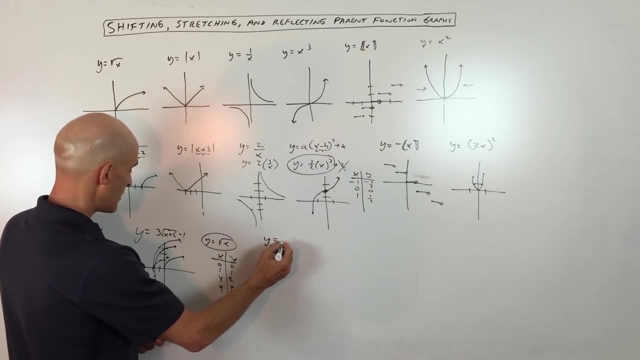 to go down one, down one and so on. so now the graph looks like that. okay, now you might say that sounds like a lot of work, right? so let's do it another way. so this is another way that students and teachers will approach it. they'll say: 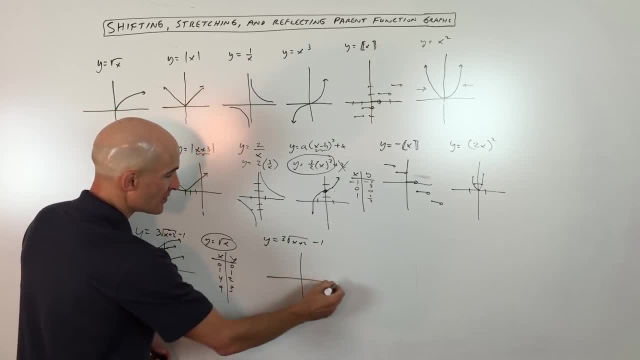 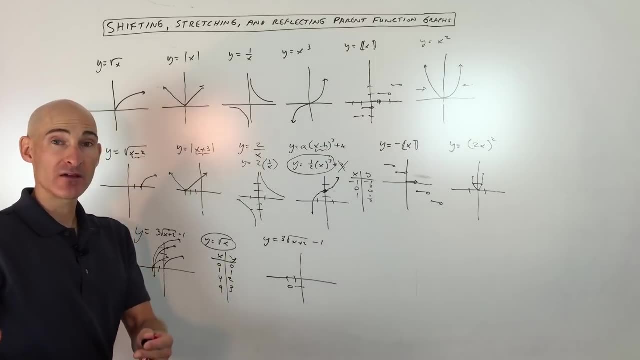 hmm, let's just take the shift into account first. let's just say, okay, we know this is going to shift left two and down one right. so let's just treat that point like our starting point, like our origin. so we've taken those guys into account. now all we have to do is graph this kind of core graph or core equation. 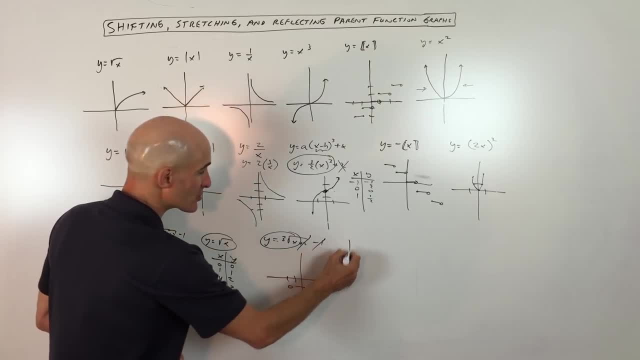 or core function, but from this point, not the origin. that makes it a lot simpler. so you make a table again. pick some easy values that you can take. the square root of zero, one and four. square root of zero, zero times three is zero. square root of one is: 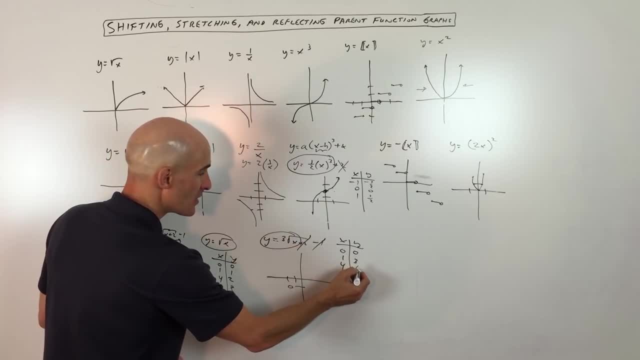 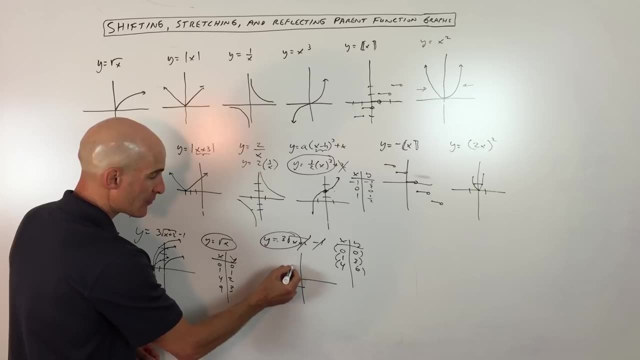 one times three is three. square root of four is two times three is six. now all we have to do is plot these points from here. so zero, zero, right, one up three, okay. and then right, four, three, four up six, okay. so you can see that this graph is the same graph that we got over here. so, depending on how your 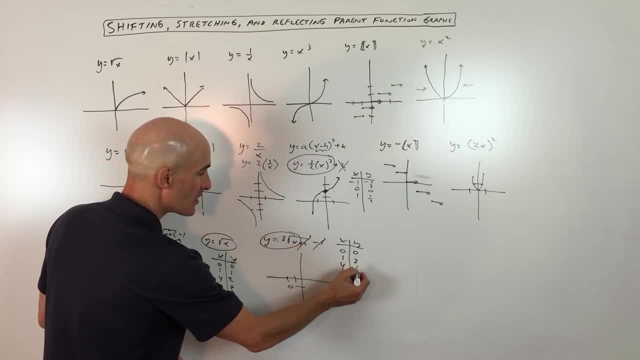 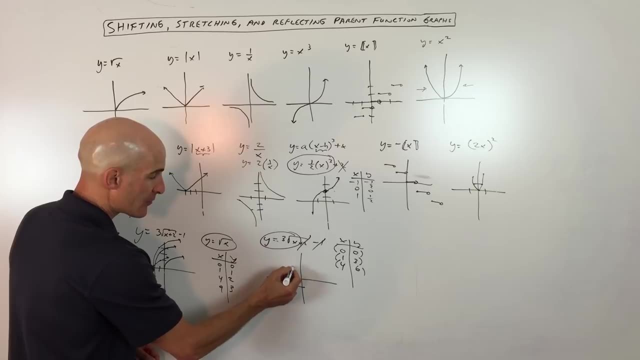 1 times 3 is 3.. Square root of 4 is 2 times 3 is 6.. Now all we have to do is plot these points from here. So 0, 0. Right 1, up 3. Okay. And then right 4,, 3,, 4, up 6. Okay, So you can see that. 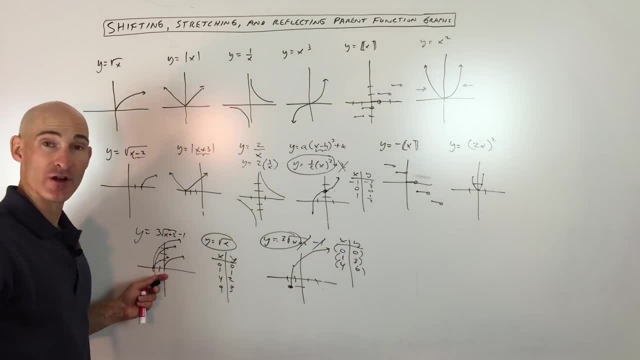 this graph is the same graph that we got over here. So, depending on how your teacher wants you to do it, if they say describe the order of transformations, you do the order of operations. you say, okay, it's shifting left 2, vertical stretch by 3, and then shifting down 1.. But if 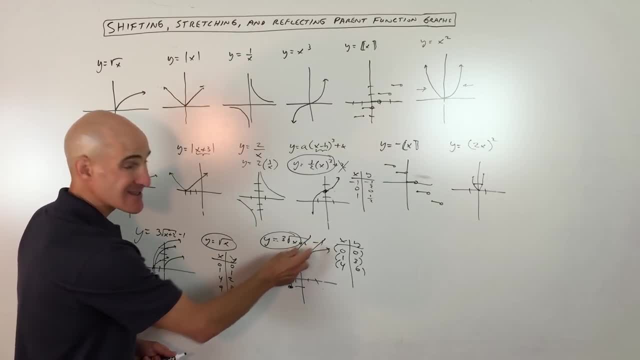 all you have to do is graph it. I would recommend doing the translation. The translation is what you're picking up and you're shifting it. That's like a rigid transformation. And then treat that like your starting point, Cover up those values that were involved in the shift And then just 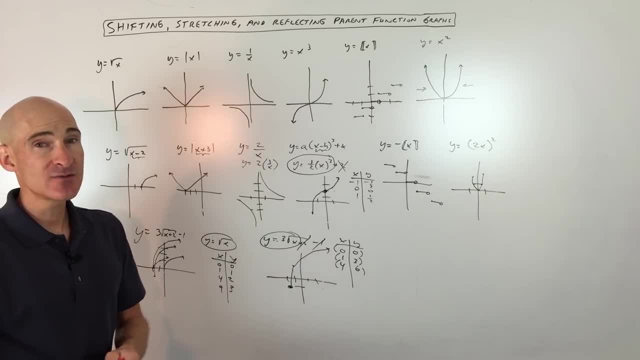 graph the core function from there. So remember adding and subtracting, pick up and shift the graph, Okay, Multiplying and dividing, stretch or compress. And the key thing to remember is that if it's graphed, you're shifting it. So if you're shifting it, you're shifting it. So if you're. 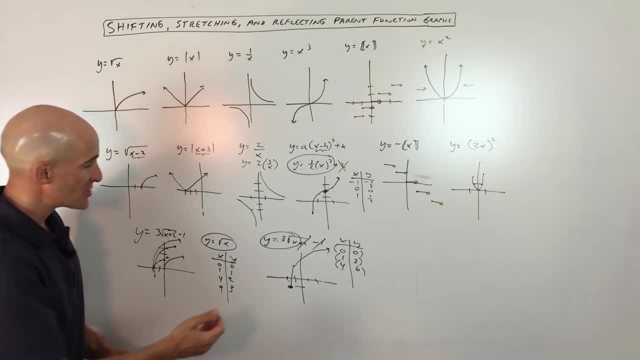 teacher wants you to do it. if they say, describe the order of transformations, you do the order of operations. you say, okay, it's shifting left to vertical stretch by three and then shifting down one. but if all you have to do is graph it, I would recommend doing the translation. the translation is what you're picking. 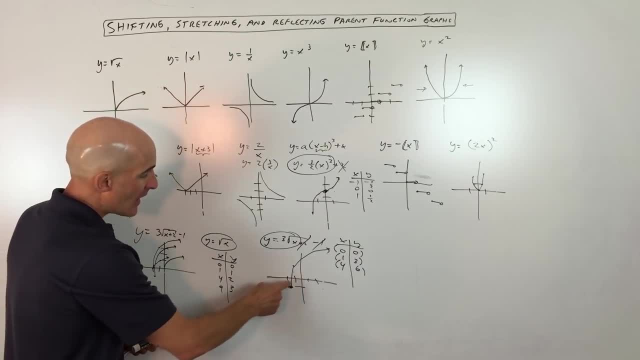 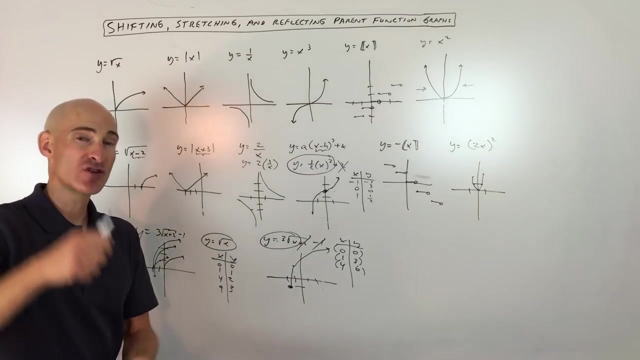 up and you're shifting it- that's like a rigid transformation- and then treat that like your starting point. cover up those values that were involved in the shift and then just graph the core function from there. so remember adding and subtracting, pick up and shift the graph. okay, multiplying and dividing stretch or 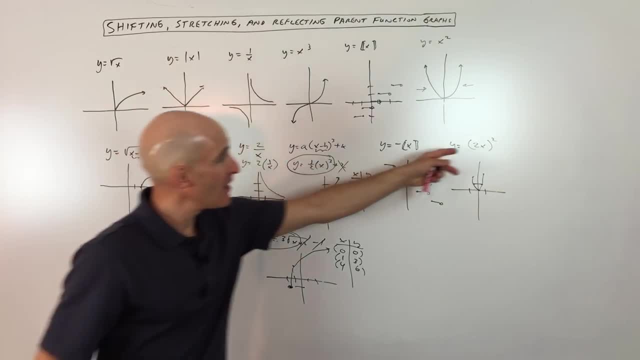 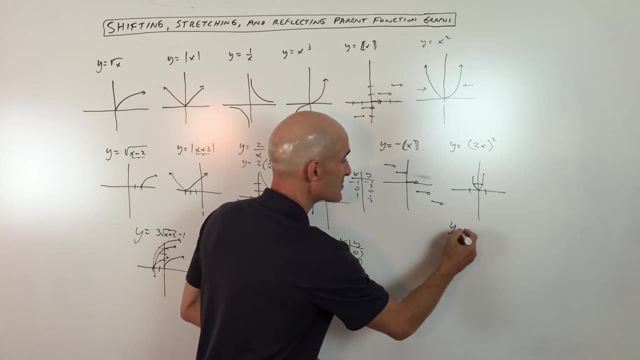 compress. and the key thing to remember is that if it's grouped with the X, it has the opposite effect. so if you're multiplying here by two, you actually divide the X coordinates by two. if you were dividing by two- say it was like this- you would actually be. 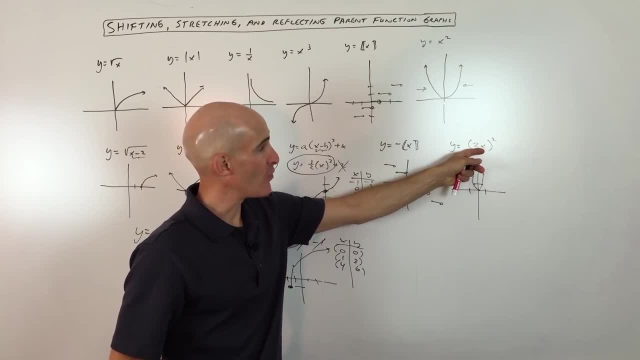 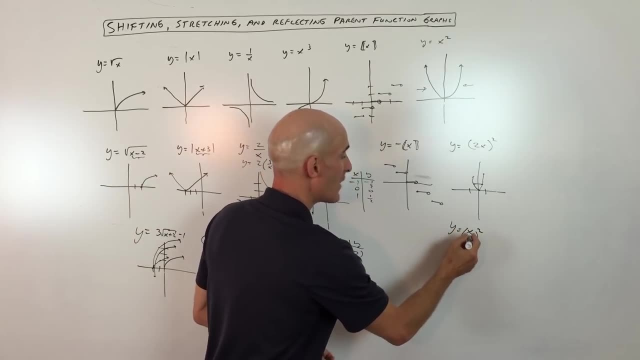 grouped with the x, it has the opposite effect. So if you're multiplying here by 2, you actually divide the x coordinates by 2.. If you were dividing by 2, say it was like this- you would actually be multiplying the x values by 2.. So it would be a horizontal stretch. Same thing with 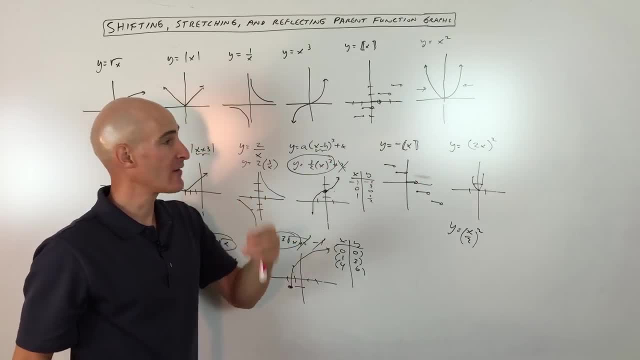 adding and subtracting. If you subtract 2, you're going right 2.. If you add 2, you're going left 2.. But if it's not grouped with the x, like say I put 1 over here, that's going to shift up 1.. If I 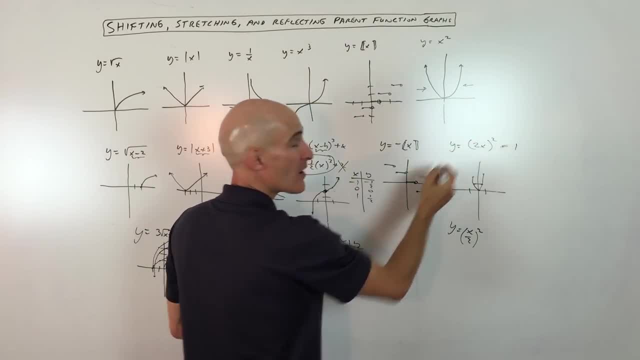 change it to minus 1, it's going to shift down 1.. If I put a 4 in front, that's going to be a vertical stretch, Okay, Affecting the y values by multiplying by 4.. And if it's a half, it's going to be. 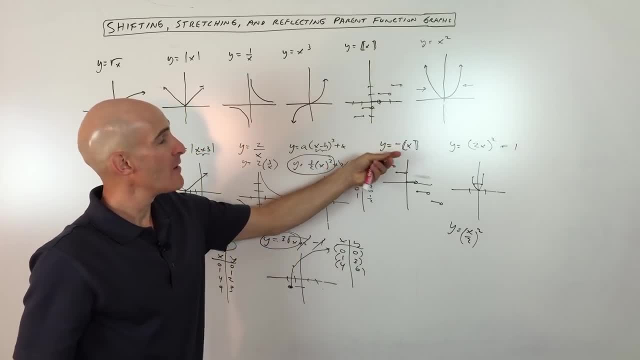 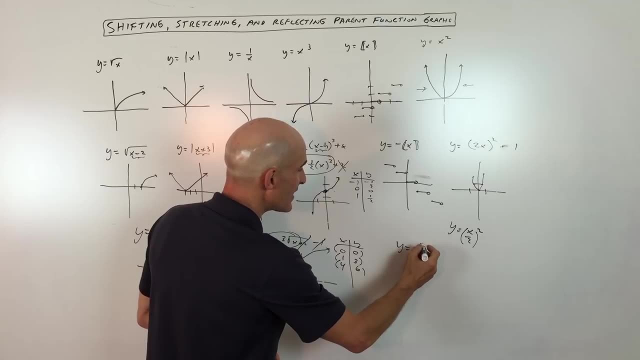 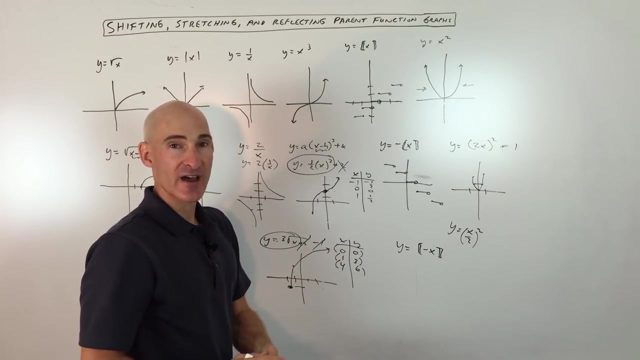 compressing it vertically. And then the last is: if it's a negative, it's going to be reflecting over the x-axis. Now one last one Bonus tip right. Say, for example, it's like this: y equals negative x. Now see how that negative is grouped with the x values. Okay, With the x. 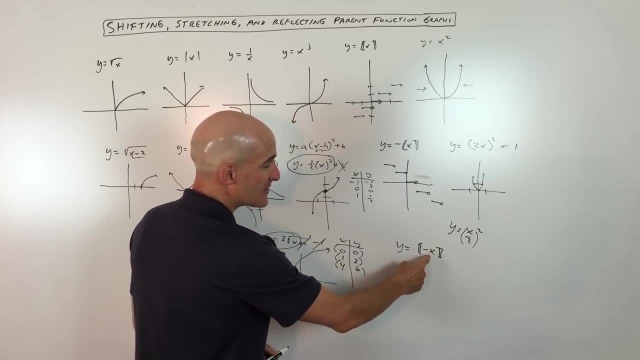 this is affecting the x values. It's making all the x values the opposite. This is actually going to reflect over the y-axis, So it's going to reflect like this: Okay, Whereas if the negative is in front, that's going to affect. 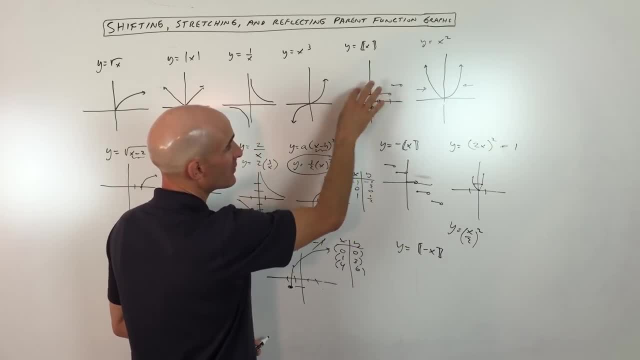 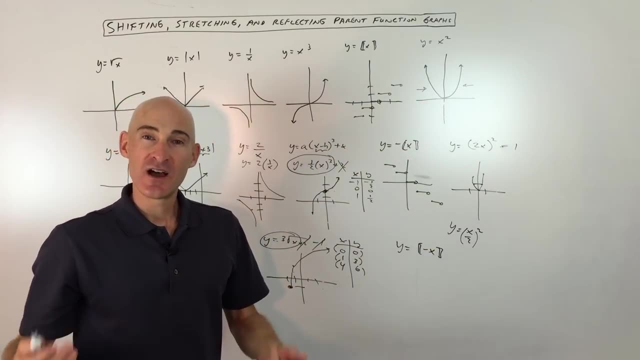 the y values. It's going to multiply all the y values by negative 1, and it will reflect it over the x-axis. So a lot of information here. Start by really learning the parent functions and then go from there. So this concludes this video. Subscribe to the channel. Check out some of my other videos. 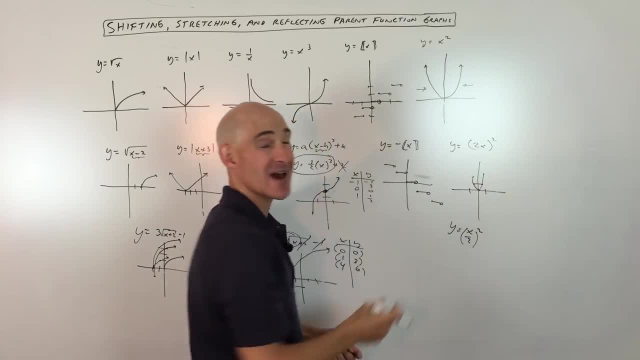 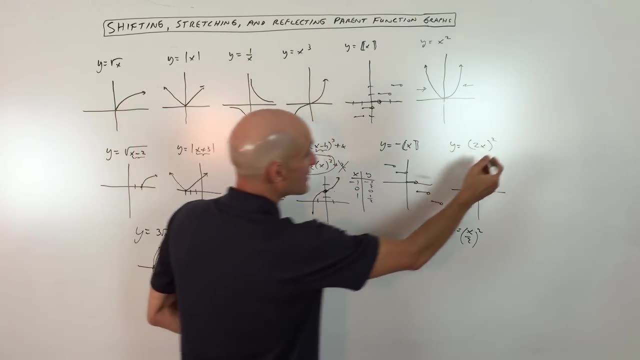 multiplying the X is about the X values by two. so would it be a horizontal stretch? same thing with adding and subtracting, like if you subtract two you're going right to, if you add to, going left to. but if it's not grouped with the X, like say, I put one over here, that's gonna shift up one if I change it. 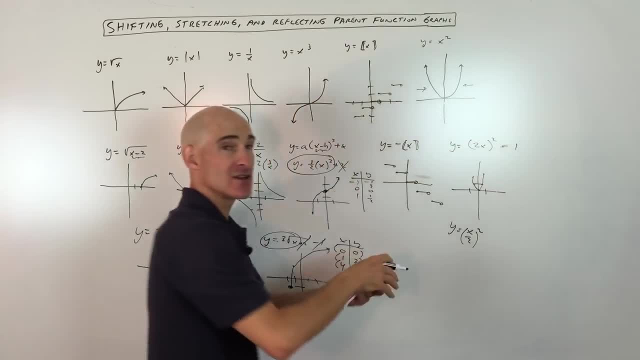 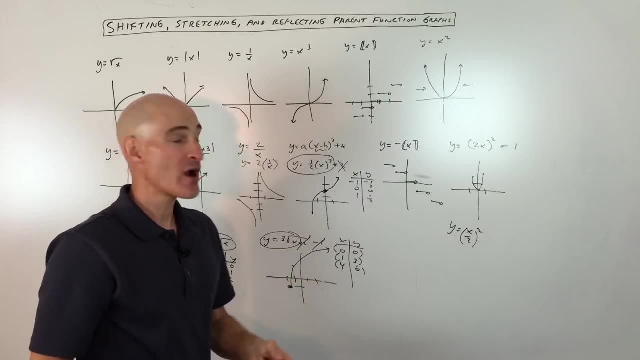 to minus one, it's gonna shift down one. if I put a four in front, that's gonna be a vertical stretch, okay, affecting the Y values by multiplying by four. and if it's a half, it's going to be compressing it vertically. and then the last is: if it's a negative, it's going to be reflecting over the x. 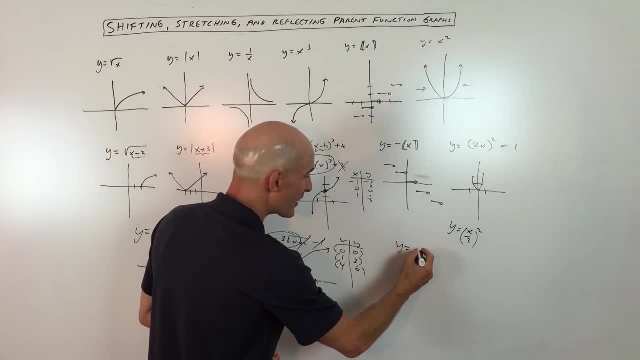 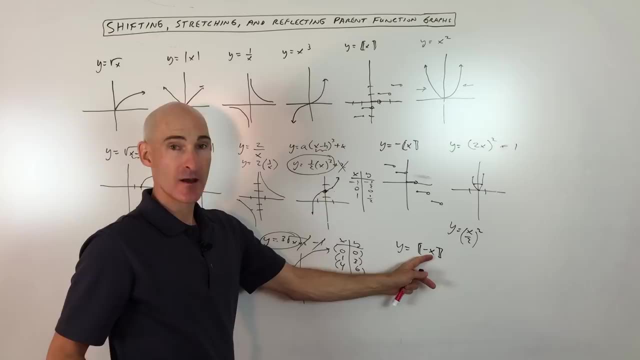 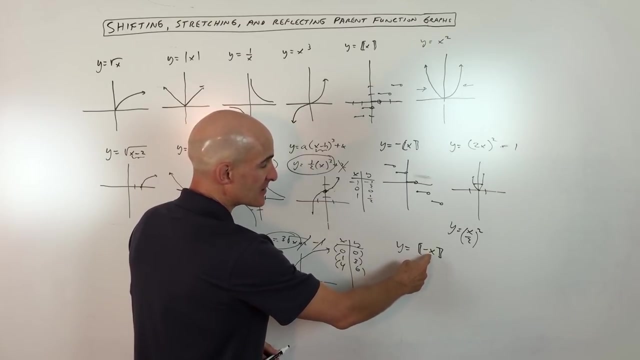 axis. now, well, mass, one bonus, tip right. say, for example: it's like this: y equals negative x. now see how that negatives group with the x values, okay with the X. this is affecting the x-values, it's making all the x-values the opposite. this is actually going to reflect over the y axis. so it's going to reflect like: 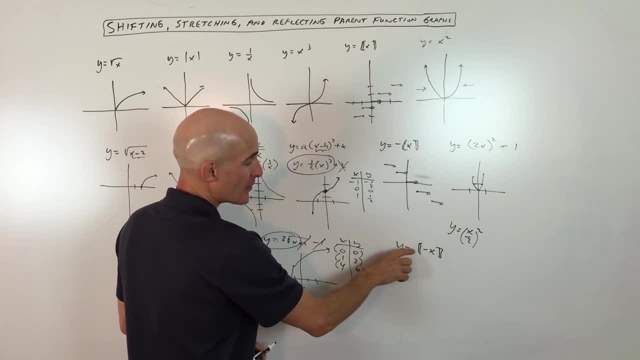 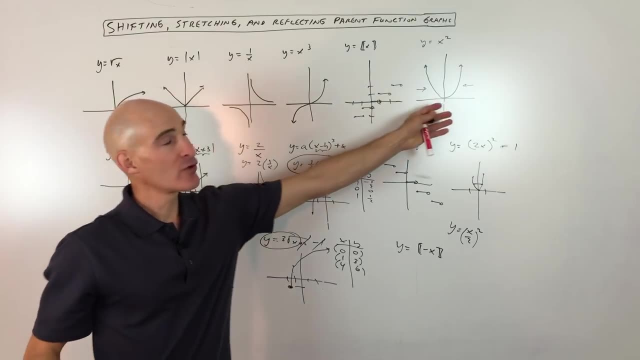 this okay, whereas if the negatives in front, that's gonna affect the y values is going to multiply in the middle all the y values by negative one and it would reflect it over the x-axis. So a lot of information here Start by really learning the parent functions and then go from there. So this concludes this. 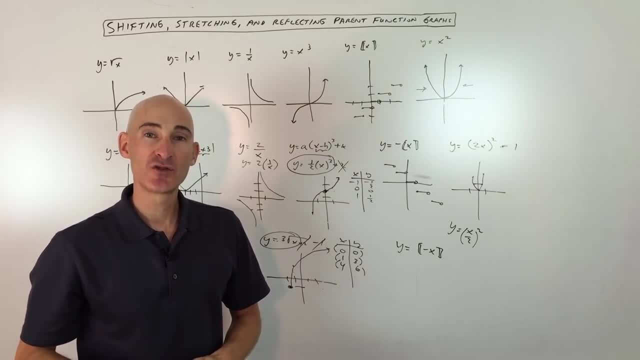 video. Subscribe to the channel. Check out some of my other videos on Mara's Math Tutoring YouTube channel and I look forward to helping you with your math in the future videos. I'll talk to you soon. 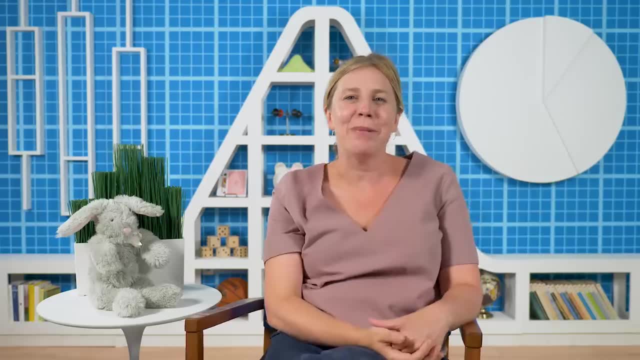 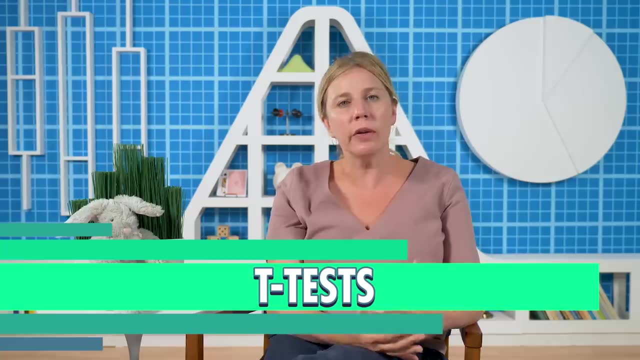 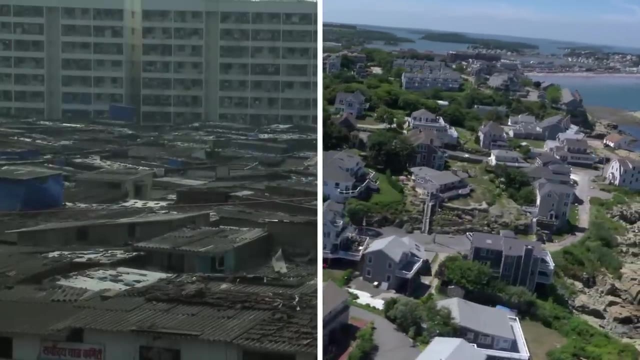 Hi, I'm Adriene Hill and welcome back to Crash Course Statistics. In many of our episodes we've looked at t-tests which, among other things, are good for testing the difference between two groups Like people with or without cats, families below the poverty line and families above. 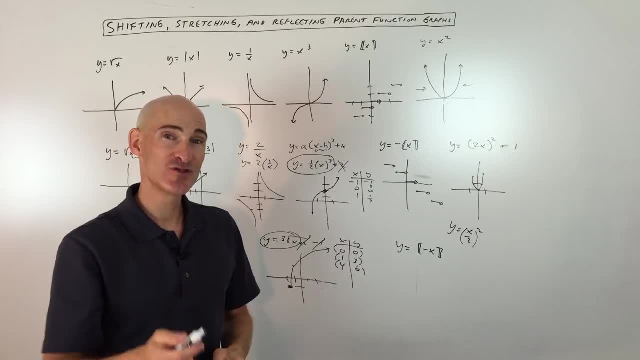 on Mario's Math Tutoring YouTube channel And I look forward to helping you with your math in the future videos. I'll talk to you soon.